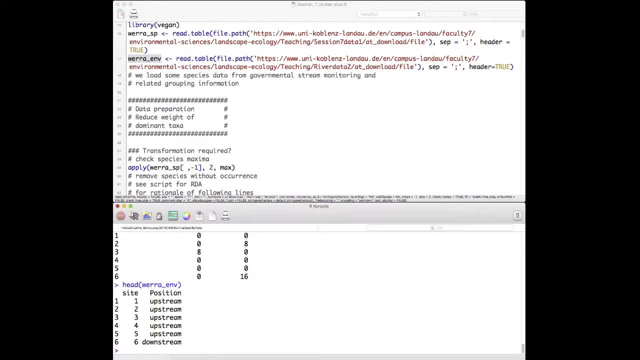 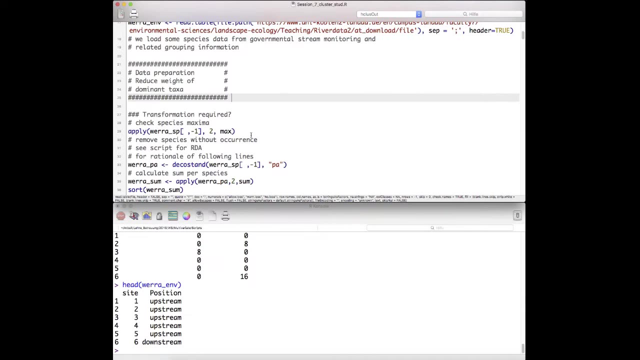 Let's have a look And at the environmental variables. here we only have the site characteristics and the position And this can later be used for external validation in the clustering data set We have discussed in the context of ordination and other methods before that. if we are looking at variance reduction or minimizing variance of clusters and have several variables, 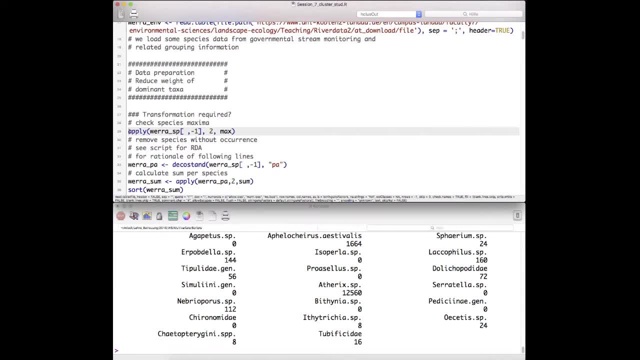 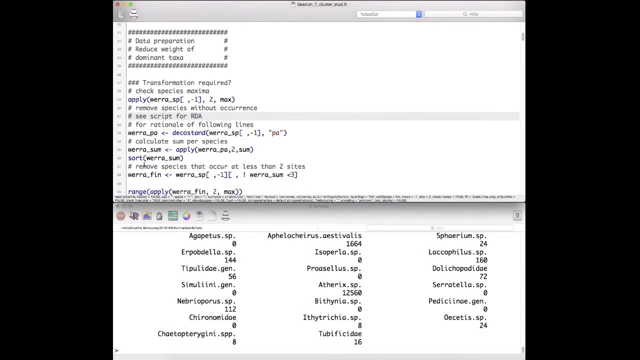 then they should be on the same scale. Otherwise, we have domination of some of the descriptors of the data set, in this case species. that will dominate the whole data set. So, as you may be used to from the previous script on RDA and PCA for species data, 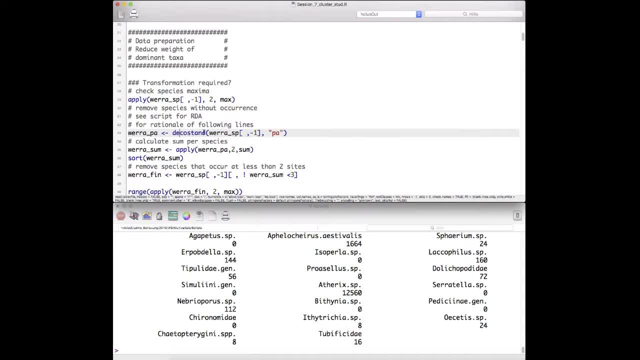 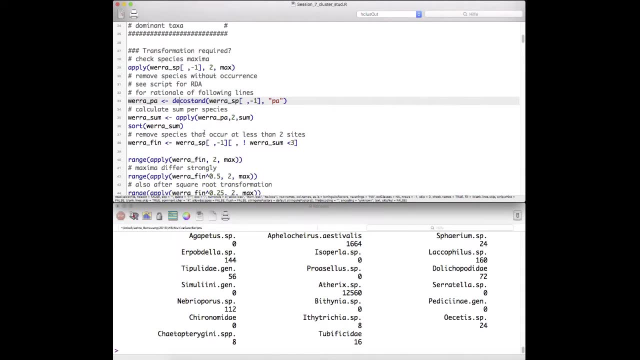 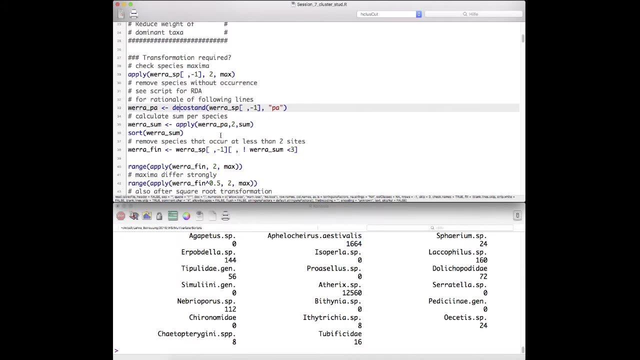 we scale this and this is done Here by later on, by first we will. we will look at the. we see we scale below here using the square root transformation and we also look at how species, how often they occur in the data set, and this is done by presence absence transformation, where we 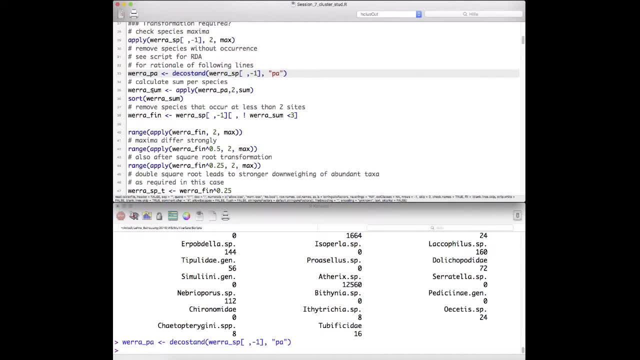 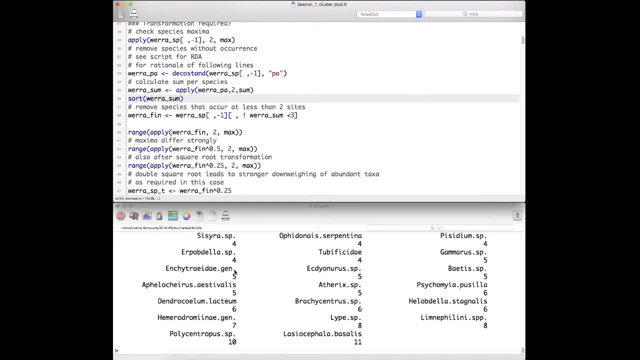 built the sum of the species to remove the rarest taxa, so this is the identical code from a previous script. i don't explain that in detail. and we sort the data and we see that we have a total of 11 sides and some species in the data set never occur, so they are leftovers. 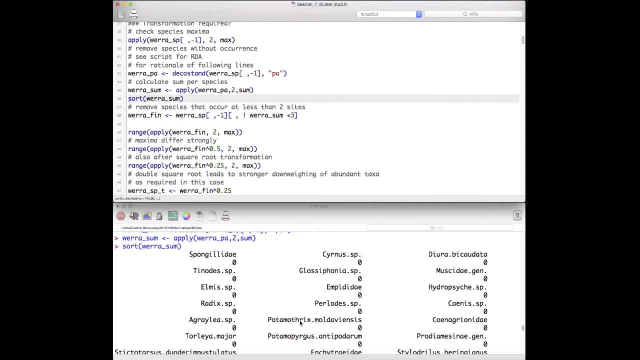 from a larger data set. these are just empty columns and we have a couple of taxi that only occur in one of the sites. now when we look at similarities between sites and we have species that just occur in one of the sites, then obviously these species will not indicate any similarity. and even with two or three sites that would. 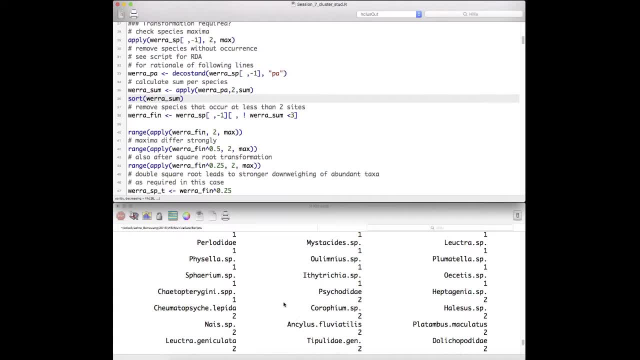 be not very high similarity with most of the sites or not be species that help in finding grouping structures. Nevertheless, we just remove the organisms here that occur at less than three sites or at two or three sites. So how is this done? We take from the species data set, we remove the first column first. 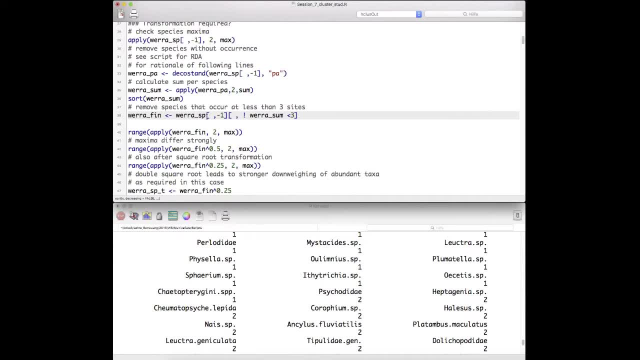 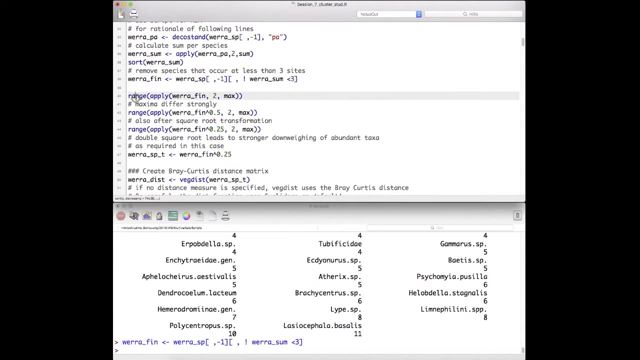 because the first column is the site descriptor. Which site do we do we look at? and then we remove the comments that had columns that have a total sum smaller than 3, so where species occur less than 2 times or less. Now we look at the range of the abundances of the species in these sites and we find 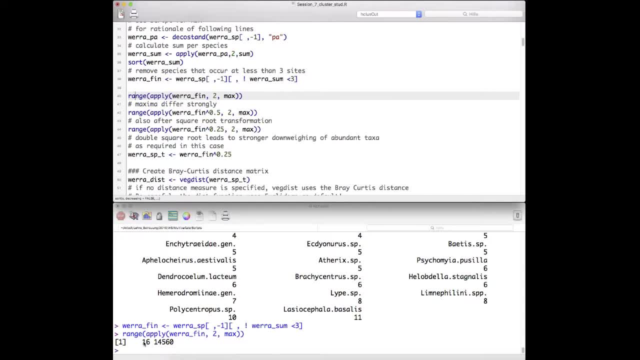 that the range of the taxa is from 16 to 15,000, so there is a really big difference in the abundances of the species in these sites. So we square root transform first and have a look at the range afterwards. So this is done. 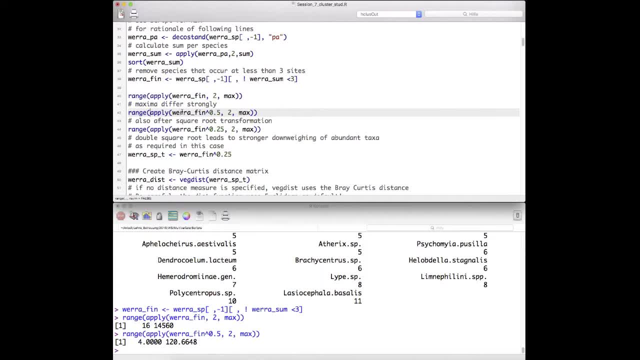 Just to explain you briefly, the apply command uses the data that is given. provided the data set that is provided here with one or two, you indicate whether you want to run a function on the rows or the columns of this data set, and then you provide the function. 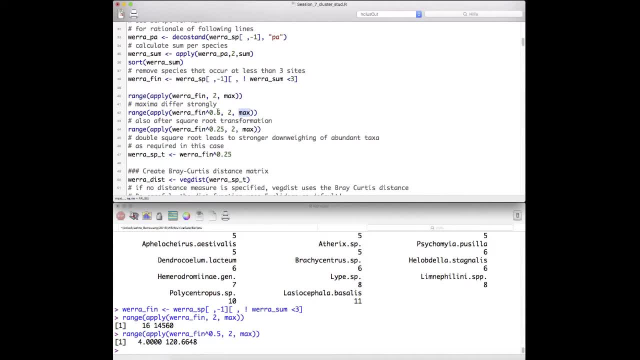 that is run. So here you calculate the maximum for each of the columns, and the range then selects the highest and the lowest value, and again we see it's now between 4 and 120, 28 or 120, and with 120 and 4, well, we still have like a factor of 20.. 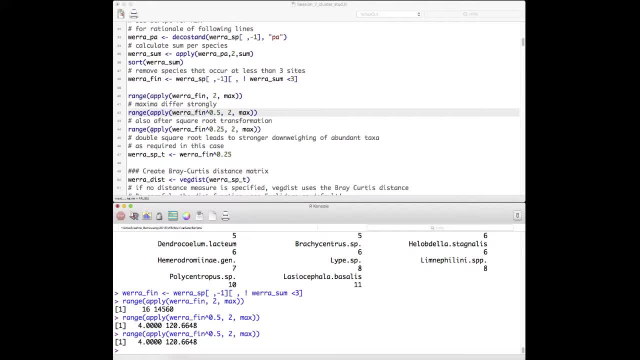 Okay, So we have a 25 difference, So we could even double square root transform and then we have the range that is within approximately one order of magnitude. So we keep, we decide here to have a strong down weighting of the abundant taxa. 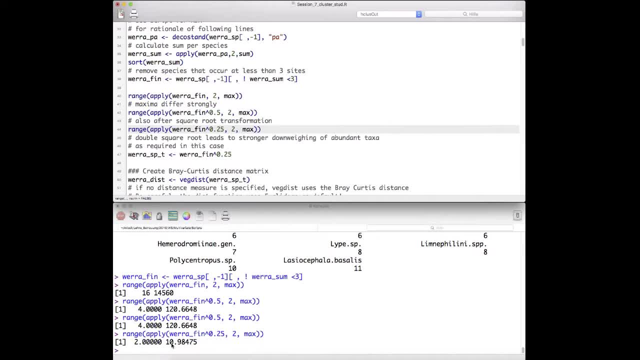 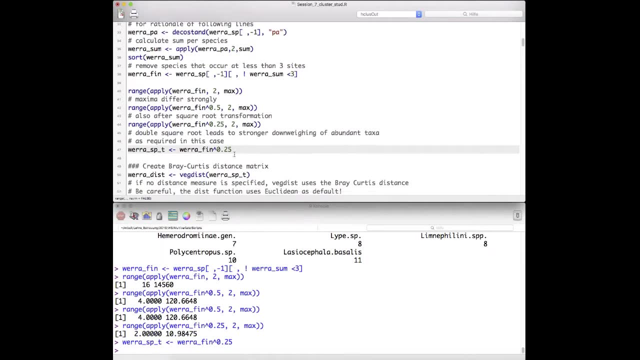 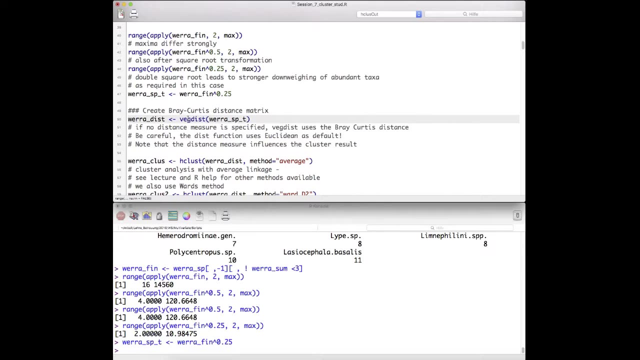 Again, this would depend on the scope of your- the scope of your research, and we transform the data into a new one. Okay, We assign it to a new object. Now for cluster analysis, we need to determine the distances and for species data we have. 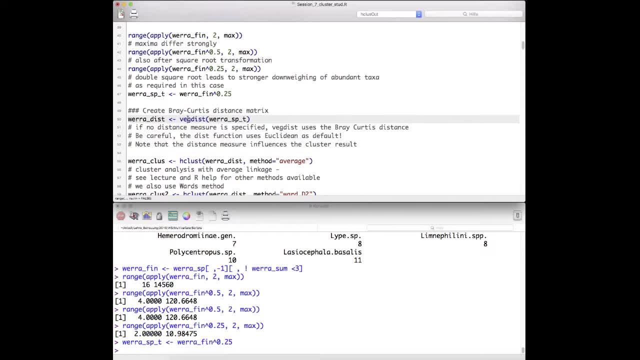 already discussed that Euclidean distance is typically not very appropriate In this case. be aware: the Vectis function of the vegan package uses the Precurgis distance that we use here for abundance data by default, whereas the dist function that is available in R uses the Euclidean distance by default. 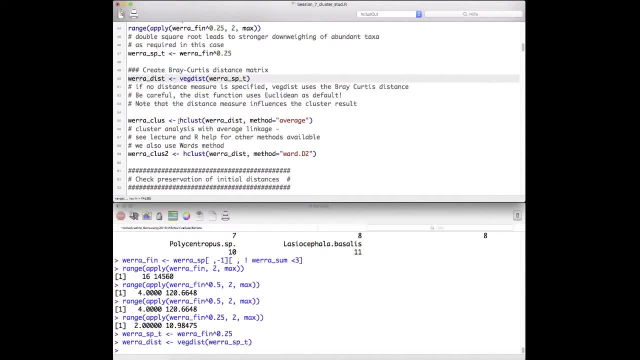 So we calculate the distance matrix and then we can do the first clustering, that we use the hierarchical agglomerative clustering. If you, if you compare to lecture, that's also the method that we started with and you may remember that there are different methods. 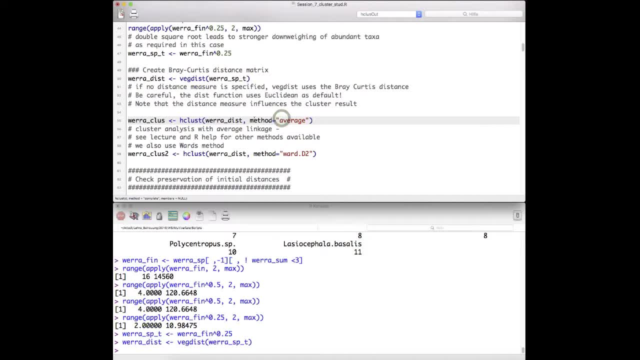 Okay, Methods that you can use. So you here, we use the average link method. There are other methods available that you are supposed to apply in the exercise as well, and they are shown. this is shown below in the exercise. the other methods on you should. 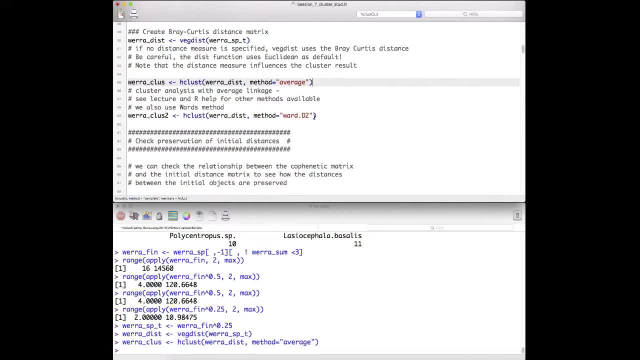 know them from the lecture. So we have the average distance here and we calculate the. we use Ward's Ward's method. that's basically minimizes the sum of squares within the, within the cluster. so it's a sum of square based method. 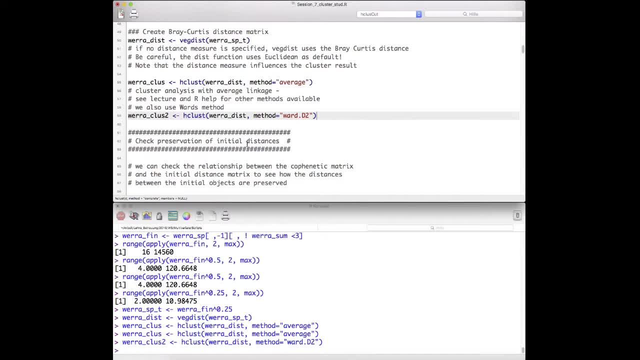 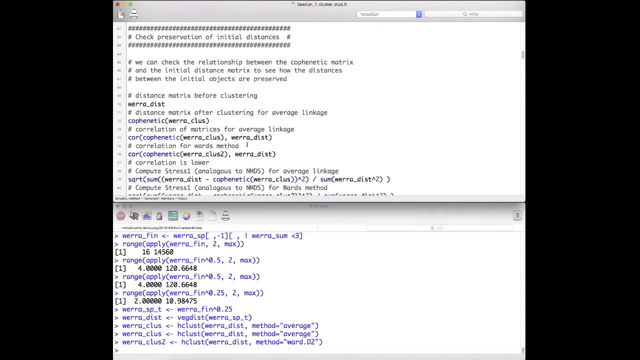 We have discussed this in the lecture already Now, when we have done calculation of some distance matrix from clustering, then afterwards or after the clustering, the all the objects will also have a distance matrix. So we can calculate the distance matrix from clustering. 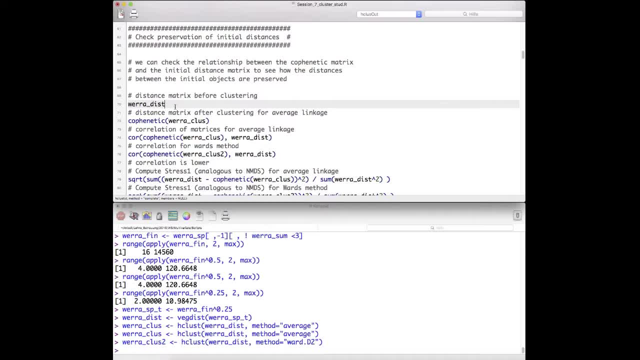 Then, afterwards or after the clustering, the all the objects will also have a distance matrix, And what this distance is is provided in the matrix of the clustering And we can take this matrix and compare it to the distance matrix before clustering. So this can help us to evaluate or answer the question: well, does our clustering algorithm? 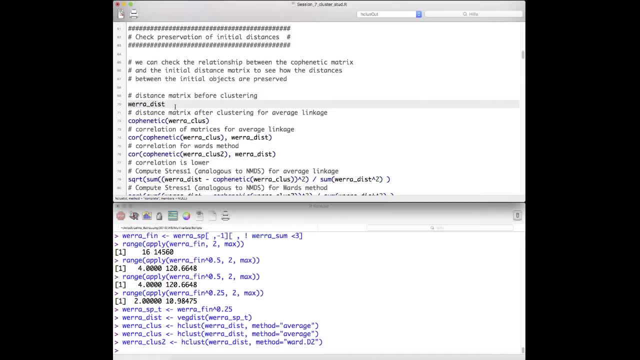 preserve, or how good does it preserve, the initial distances that we have? Well, the answer is that the initial distances that we have are the distances that we had between the objects. how they are, how are they later represented in the clustering solution? 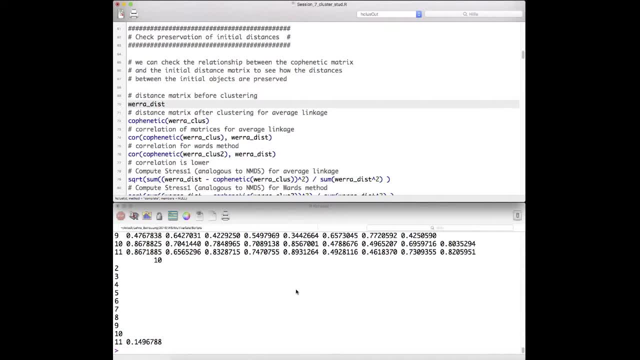 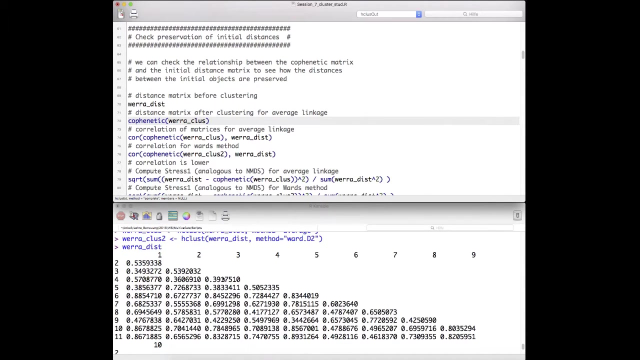 And remember that our, that our method is actually that the method that we use, average linkage is a decision how you calculate the distances between two clusters or between clusters and objects. Okay, Thank you, Bye-bye, matrix is provided. so here we have. first the distance matrix, the initial distance matrix. 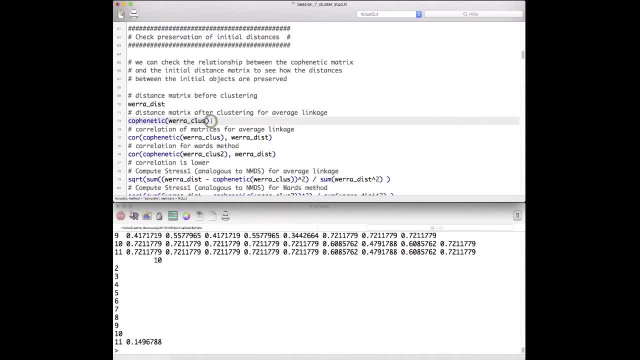 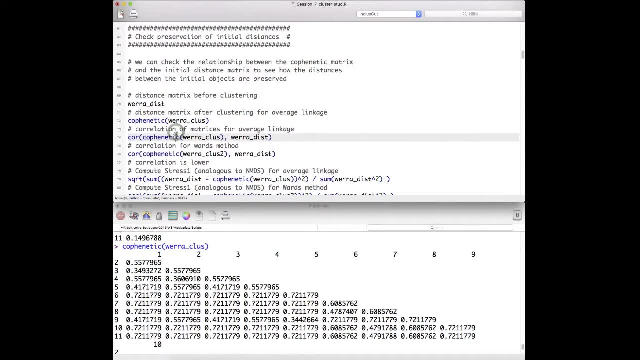 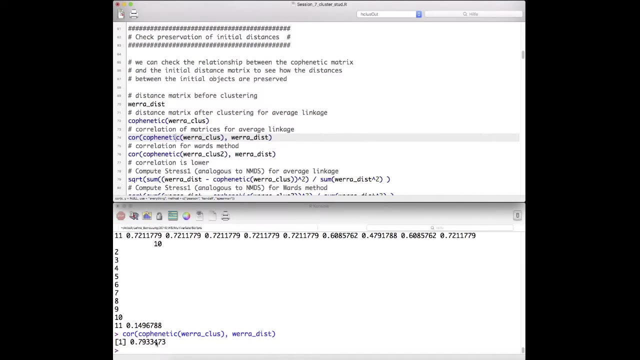 that's based on the pre-curtis distance. and then we have the cofenetic matrix provided here. that is the matrix after clustering, and we can simply calculate now the correlation between the two matrices, and we see that we have a correlation of 0.79, so 0.8 almost. 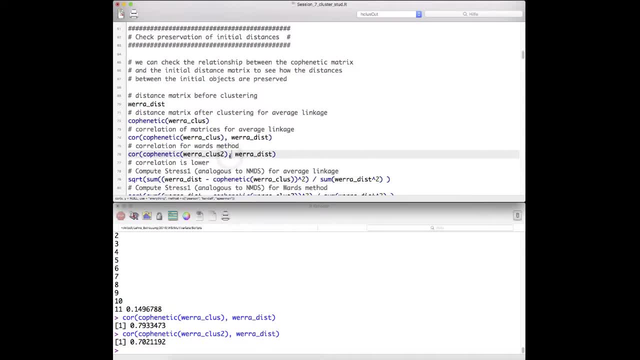 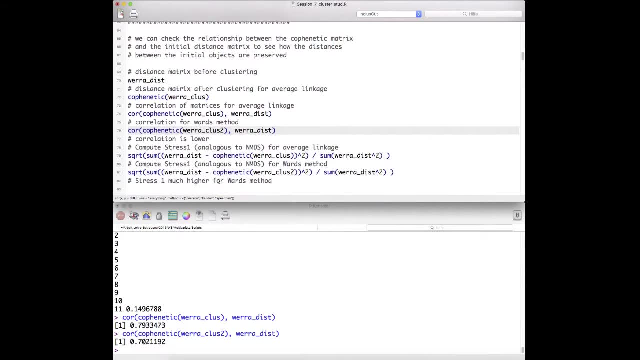 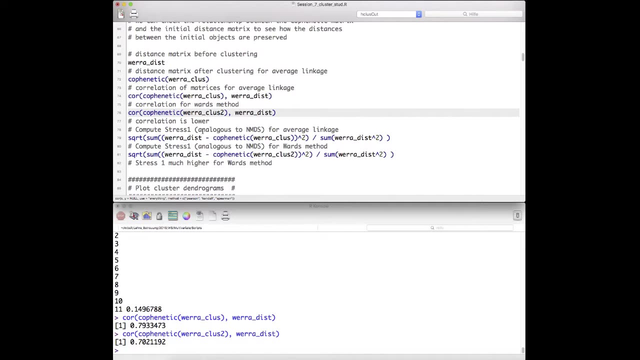 that's a relatively high correlation. if we compare this to the correlation for the ward's method, we see that the correlation is lower. we could also calculate the stress value. remember that we defined stress in the context of nmds, so it's used to to sum up the distances. 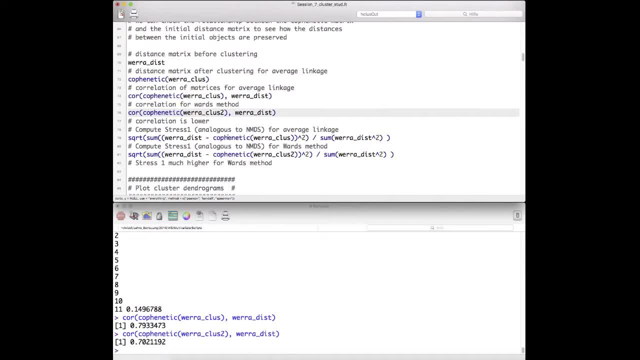 between the initial this between the initial matrix and the resulting matrix. i'm dividing this by the sum of squares. so, and remember that for the nmds, who had some, some guidance on how to interpret the representation in the resulting matrix from nmds matrix, we said: if the stress value is below, 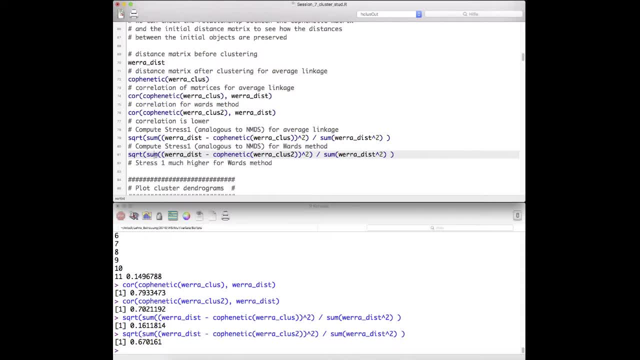 0.1, then the representation is fairly good. but in this case we have, for the average linkage we have, we have a stress value of 0.16, which is still acceptable, whereas for the average for the for the warts method we have, we have 0.67, so very high. that's not a very good representation of 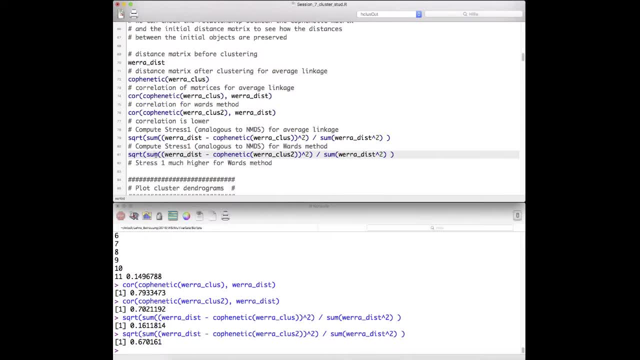 the initial data. now, keep in mind that in clustering, you are not, we may not be aiming of representation of the initial data, but we may not be aiming of representation of the initial data or representing our, our data, in a most appropriate way to most represent. we wouldn't we. 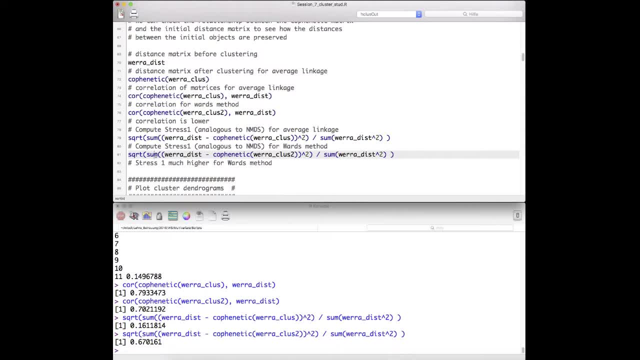 may not aim to represent the data in a most appropriate way or keep. keep the same structure. we may want to find groups or we may want to find outliers and therefore distort the data. for example, build clusters that space contracting or space delay ting. we have discussed this in the 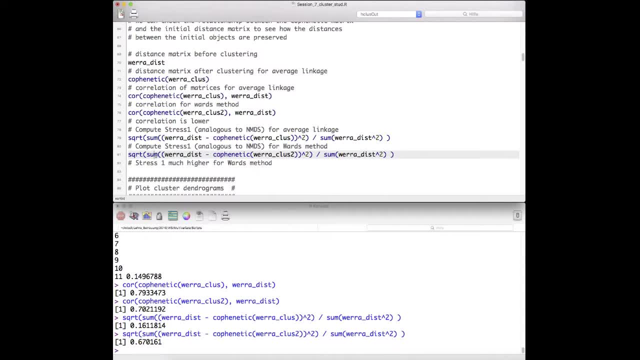 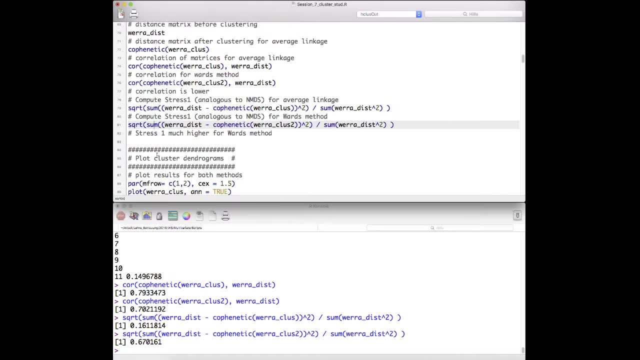 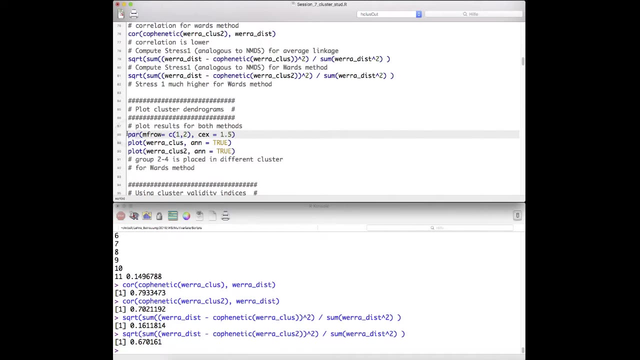 lecture. so it's not necessarily indication that you shouldn't use this clustering method here, because our aim may not be to represent, to have a representative and to have a good representation of the initial data set, because we have a different aim. so just use them if you want to know or if your 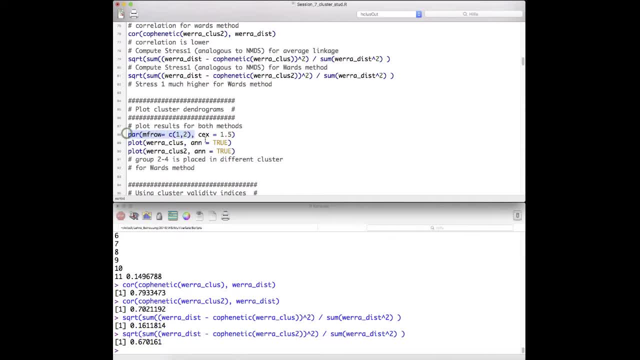 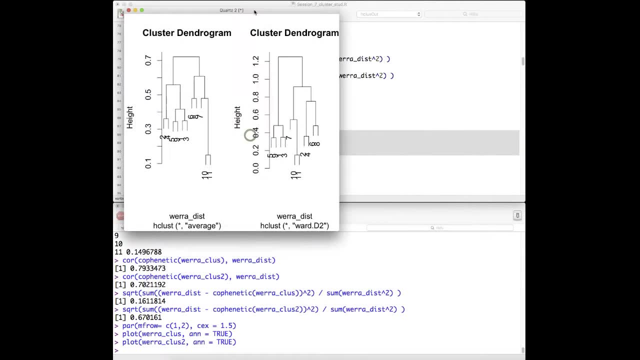 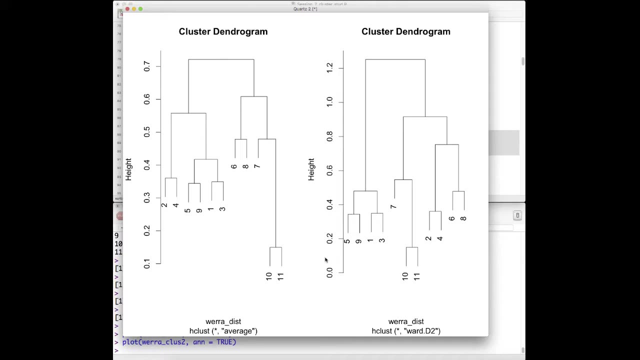 aim is to have a good representation of the initial data. we can now plot both resulting dendrograms. we have discussed briefly dendrogram in the lecture you have to hide: here that's the distance that's given along the. here it's along the y-axis. you can also. you could also turn this dendrogram in description in: 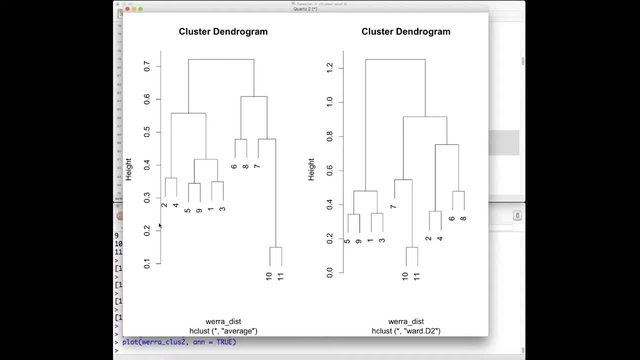 the horizontal form. let's just have a look into the function and we see here the individual sides, how they are related to each other, and you would also see the the steps, that at which step which objects are merged into a cluster. so first, side 2 and 11 are merged into one cluster. we can derive from that that 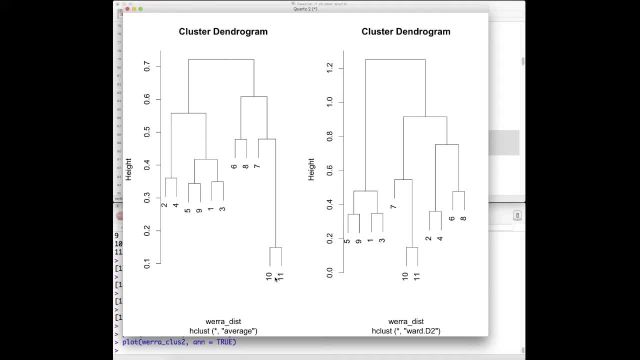 these are the most similar sides in the data sets, side data set in terms of species composition, and we see that this actually is the same for the average linkage method and for a ward. for the ward method, and we see that overall we also come up with two clusters that are relatively well. 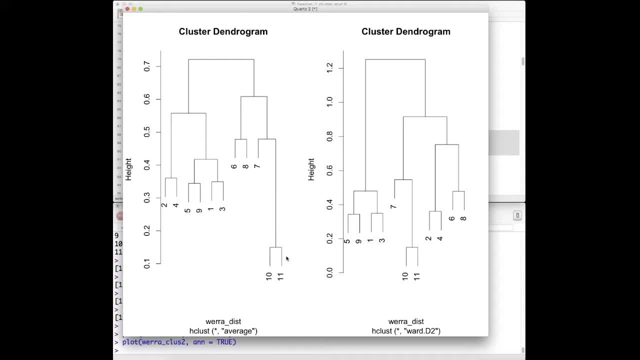 separated. so nevertheless, 2 in the 11 seem to be quite different to the side 6, 8 & 7, when the same holes on the on the left side of the side, the panel we see here, the size 24, seem to be quite different from the other four sides. 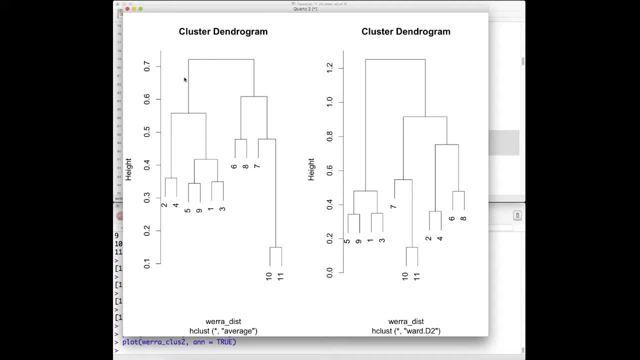 Now, how many groups do we have? we will discuss that later on. but you see here that you could cut the clustering at different points. you could cut it here. then you have two groups- you could make a cut here. then you had four groups- you could make a cut here. then you had actually a couple of. 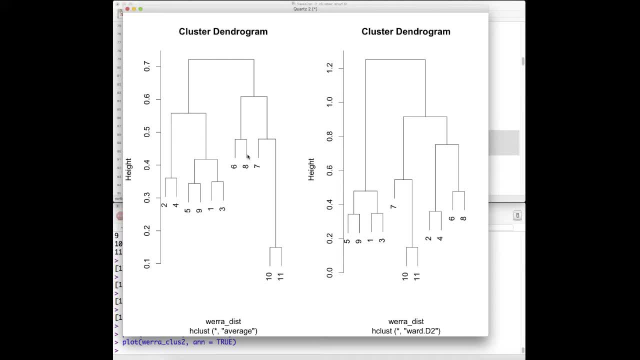 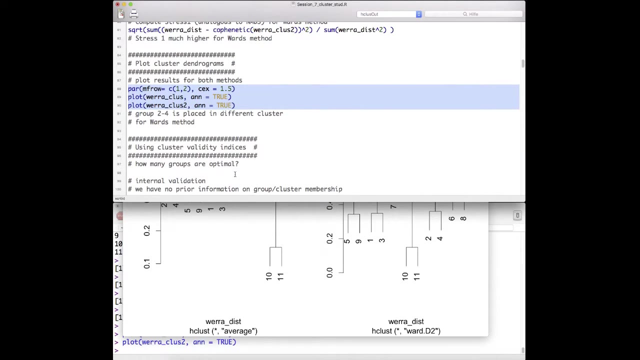 of sites in the singular clusters and single clusters and so on. So it's not straightforward how many groups you have, but the visual representation of the data may guide you in evaluating how much classes you want to have. Remember it's an exploratory method. 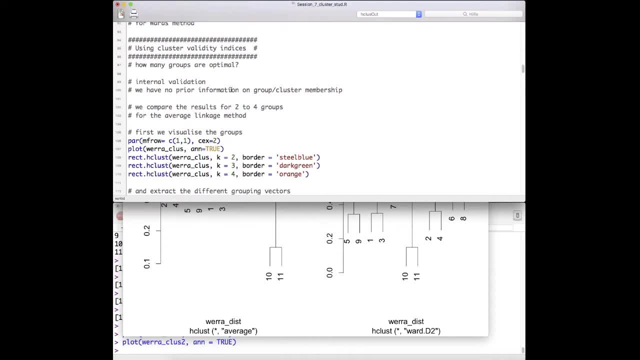 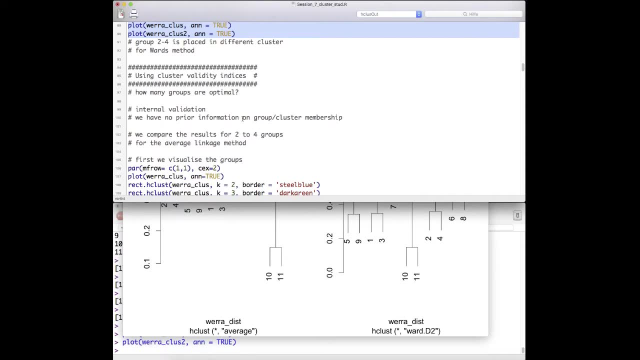 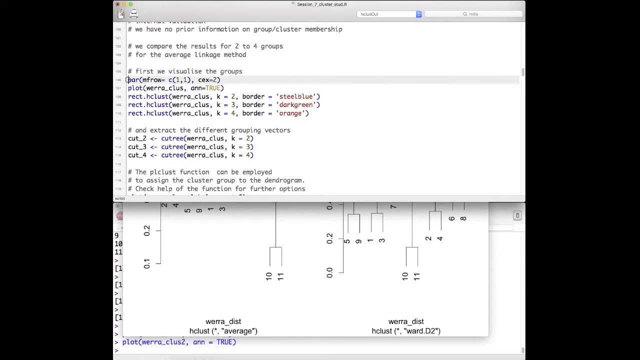 So we will use first and we will, let's say, we had a look at this and thought: well, two to four classes may be appropriate and we want to calculate cluster validity indices for that. We do this first. before we do this, we visualize the groups in the in the clusters, how this would 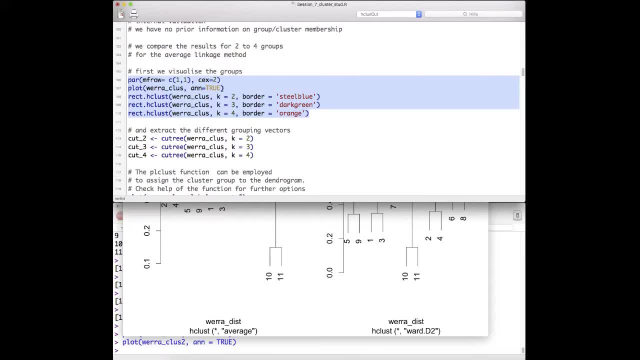 look like. So we plot here the cluster. again annotated true means that we indicate the sides and then with recthclust and then providing the data set and k. as you may know from the lecture, k always defines the number of clusters. Here we can indicate in the plot where the plot would be cut, where the data would. 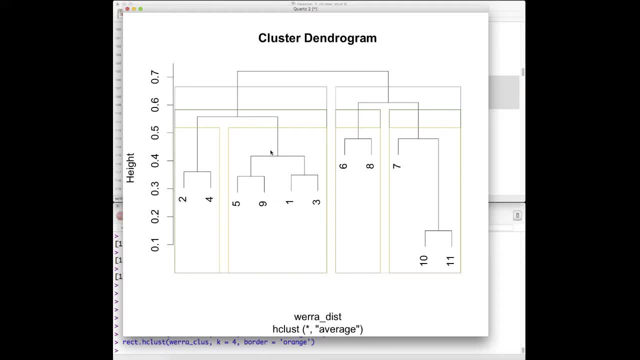 be cut to define groups. So we see here: for k equals 2, the two blue squares indicate the two resulting groups with k equals 2.. So k equals 2, k equals 3.. You had the green groups indicated, so that would be one group. 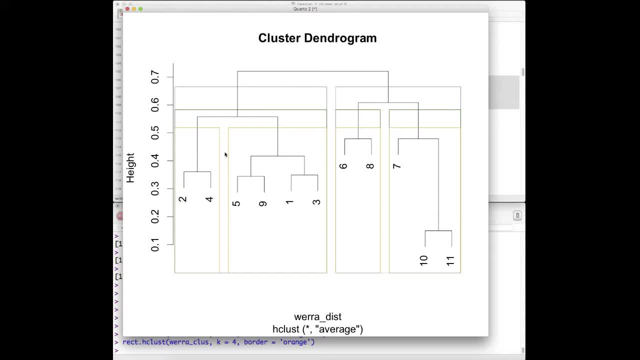 that would be one group. six and eight and seven, ten eleven would be one group, and with yellow indicating four groups. this would be the groups two and four, Four, nine, one, three, six, eight, seven, ten, eleven, And the resulting partitioning is called the clustering. 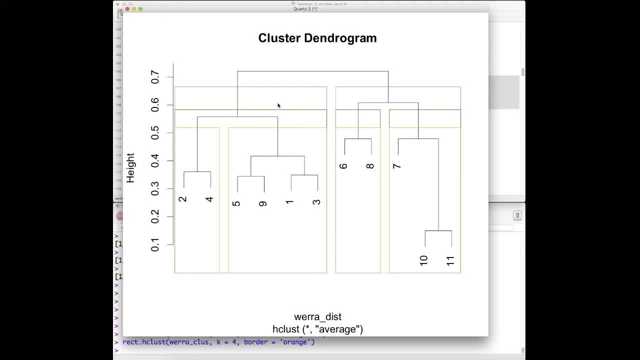 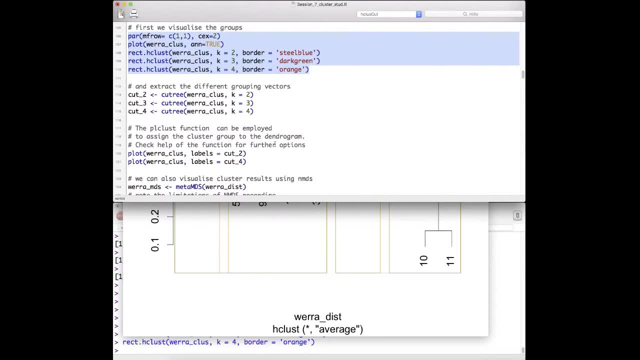 So what you obtain from this is a cluster structure. the clustering is a vector that assigns the group number or the cluster number to each of the sides and that can later be used in evaluating the clustering. So to do this, we to obtain this vector, we cut, we use the cut tree function, cut tree function and where it should be, how many. 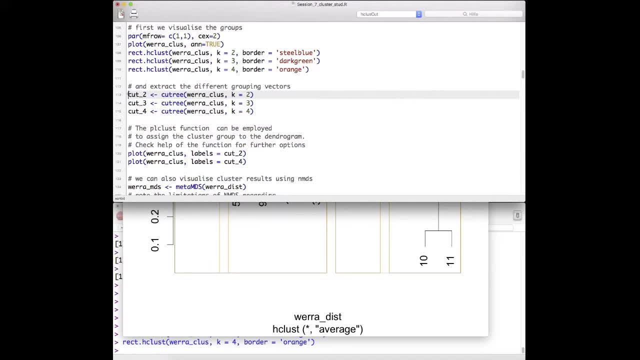 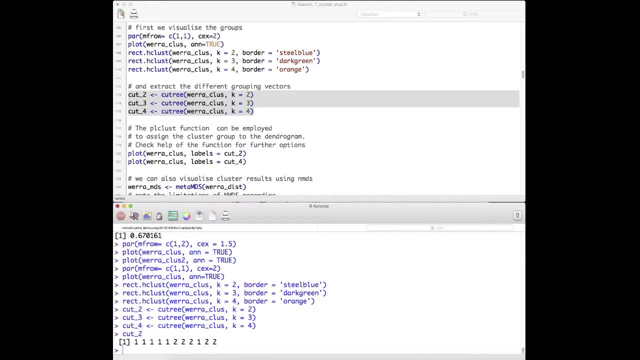 resulting groups. you want to have how many clusters? and when you cut this, the object that you obtain- just let's have, let's have a quick look- is just a vector that assigns a cluster number to each of the, to each of the sides, to each of the objects. 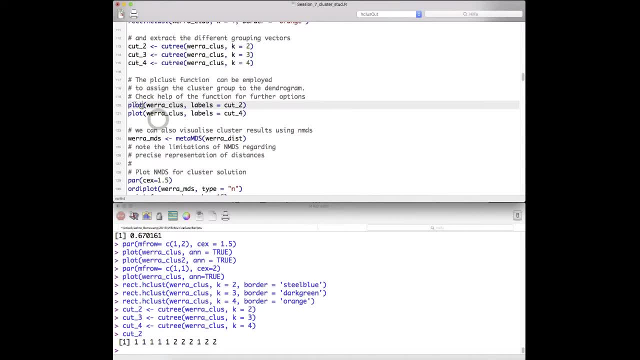 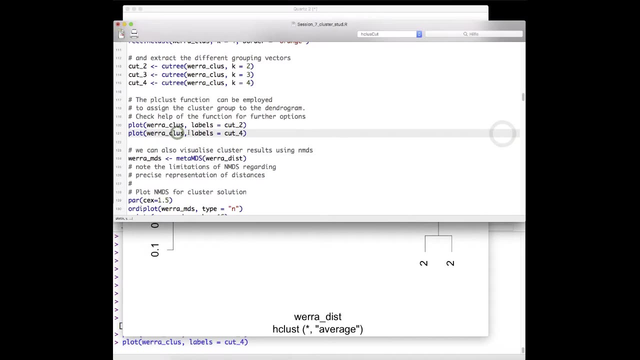 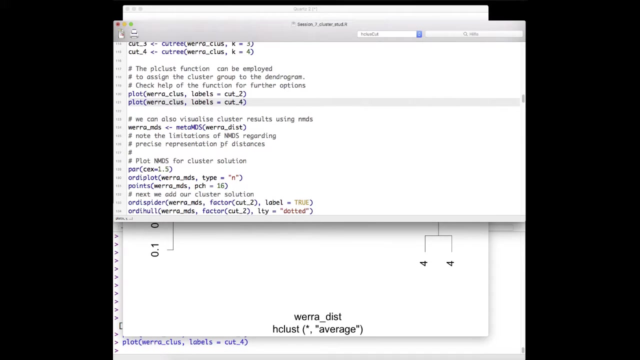 in the data sets. We could now use this vector and plot the data again. we could now use this vector and plot the data again, and plot the data again and assign the cluster number and do this for two and four classes. so that's pretty easy and just a final why to visualize or a final method of 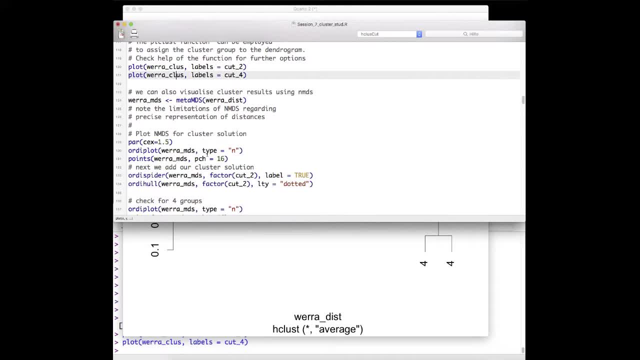 visualization is to use the NMDS that we've discussed in the previous part of the course. so we don't define, we just use the function wrapper. we've discussed this method, that this contains a lot of sub methods that are used and, pray Curtis, we in the use the distance metric directly in the function. and what? 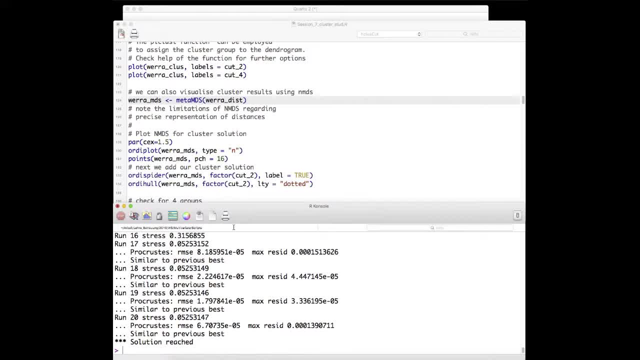 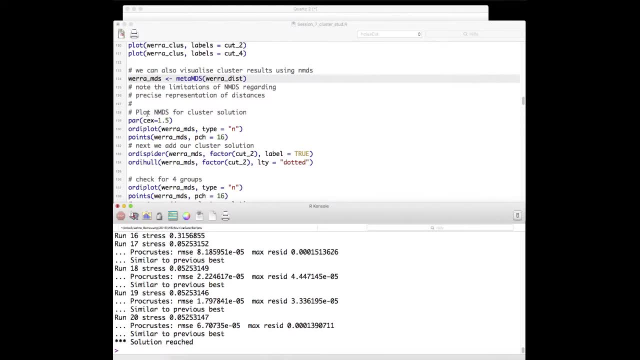 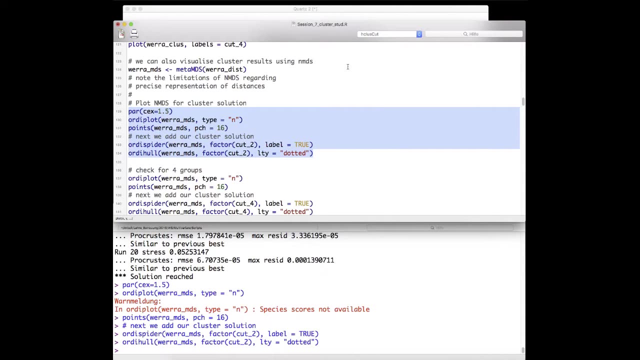 we can. what we see here is that we have relatively low stress value. so point zero, point zero five. that means we obtain a very good representation of the data and we can now plot the data for the two clusters. so if you're looking to the code, we first create the plot with type equal n. that means that we don't want to. 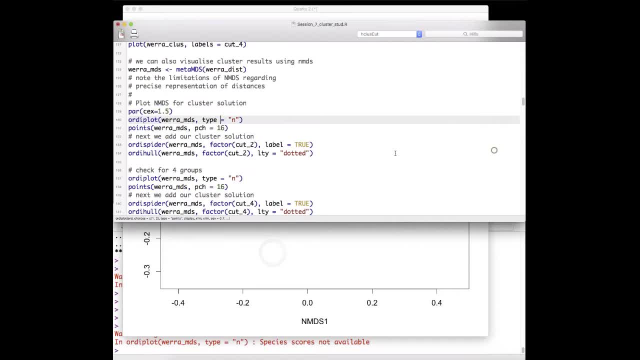 just do this again, that we don't plot. so we don't plot anything initially. then we plot the points. so that's happening here, and with the function or the spider you provide the data set, you provide the factor, the factor, a factor level that is used to assign different groups. so cut. 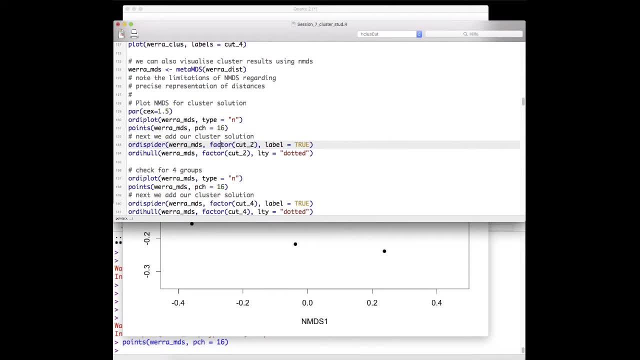 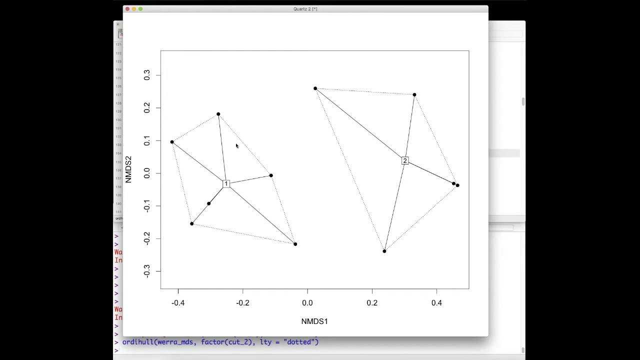 two is just a numeric vector. we need to convert that to a factor. when you do this, it creates this kind of spider, so it connects all points to the center of the data, to the grouping here, and or the column creates the hull around the individual clusters, so that's displayed. 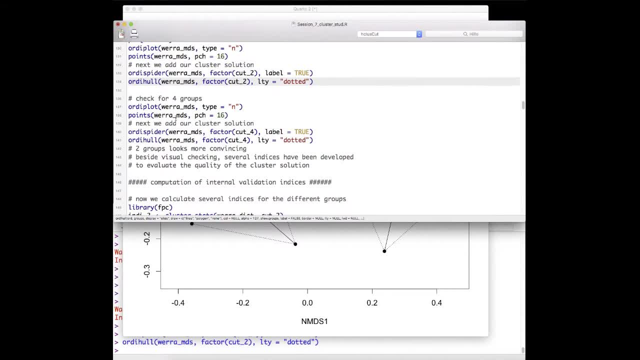 here. so that looks like quite nice and gives you an indication we can do. we could also do this with four groups, or the code remains the same. we just used a grouping vector for the from from the edge for the cut tree function with four groups, and then we obtain something like this and then we get the value of the. 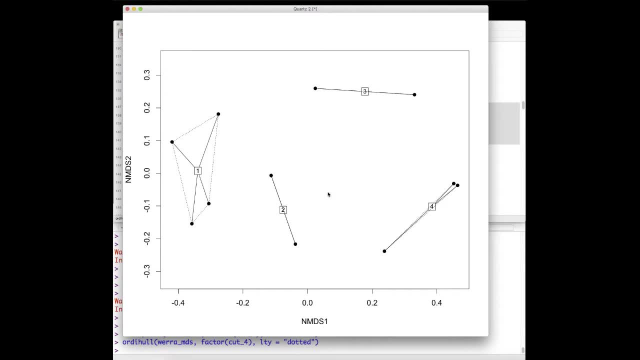 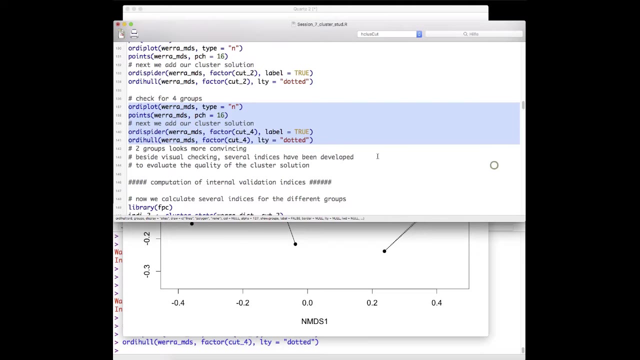 two groups. another way that's explained is that, as we say, in a picture, we can beских to the right side like this, and then we see that the spin is actually a minimum of two points. and that's an education, let's say. we can see that, we say that we are starting with an extra point from a point and 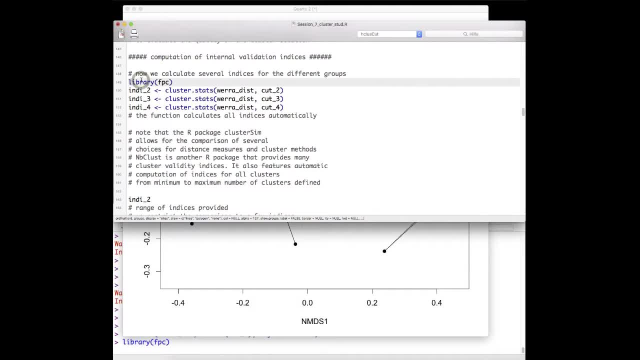 then we calculate some internal validation indices. these are cinematics which we are supposed to do in the next video, and then we will talk about it. the in the library FPC The function is called clusterstats, and this function actually calculates a whole range of internal and 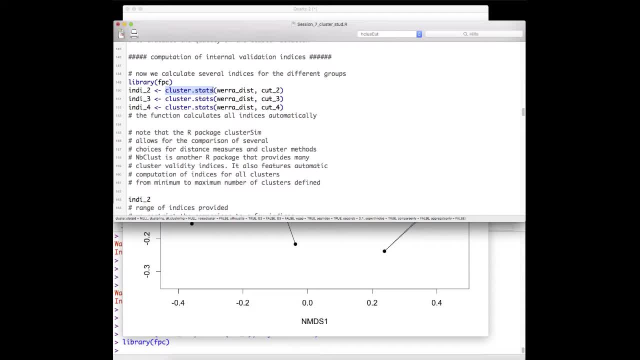 external validation indices and we- but I don't want to go into details of it- into each of the several indices that are computed. Theoretically, you could also use something that is called a voting scheme, where you add up the way you try to integrate the different indices by, for example, if, if, 10 each. 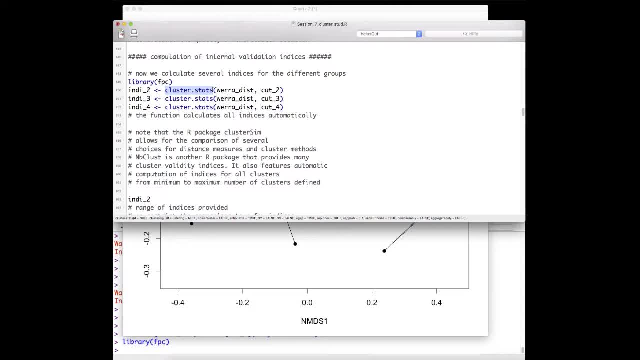 each of the index votes or the result of that. what is an optimal number is a vote for a certain grouping structure, and then you will calculate how many indices resulted or voted for a certain number. You can take the number of groups and take the maximum of this vote or. 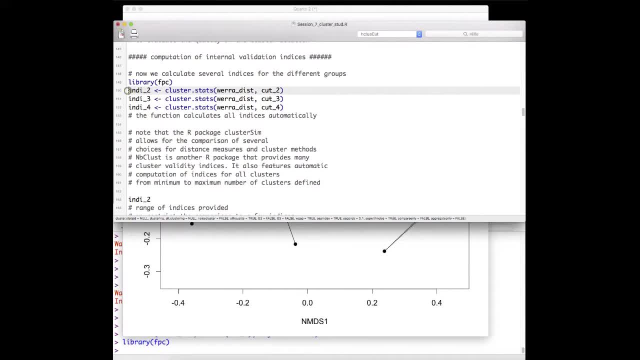 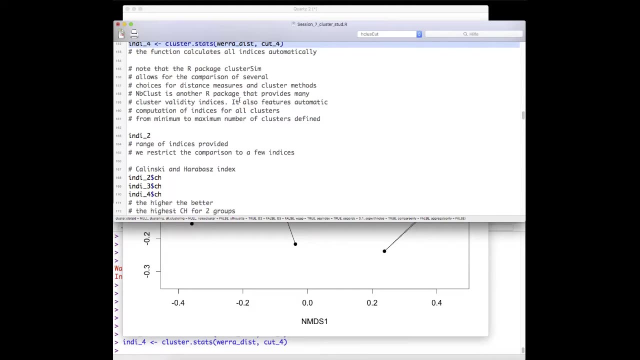 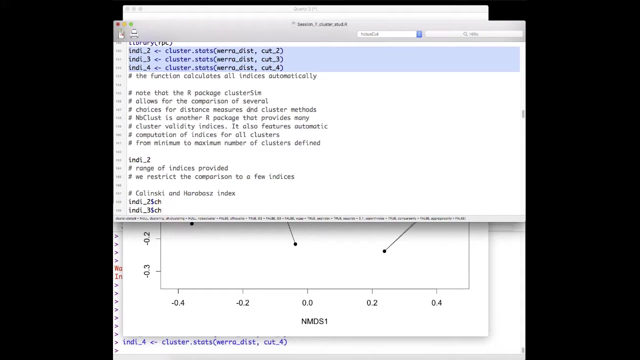 something like that, but have a look into the literature. that's beyond the scope of our course but could be done with this method. So we calculate the indices for two, three and four groups. Read this text here. There's also the cluster sim package where you can provide different clustering methods and different groups. 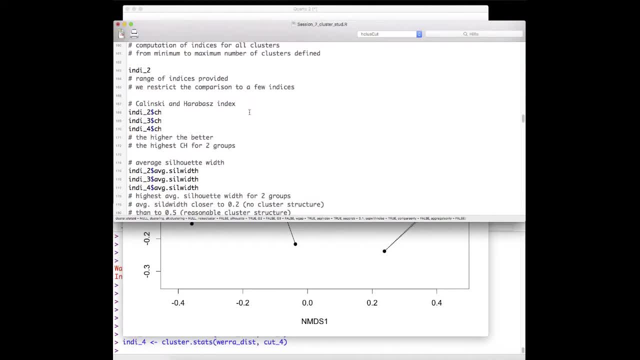 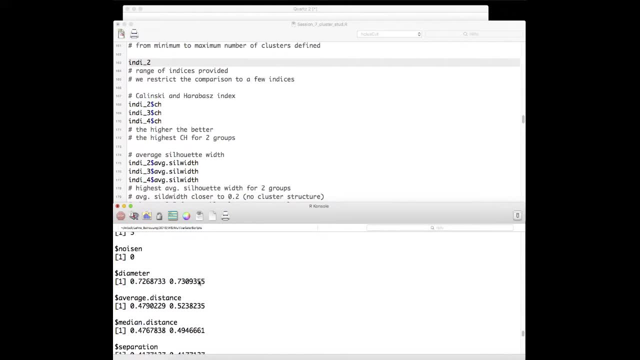 that are calculated automatically and we quickly have a look at the different results. that what the object contains. So it contains a lot of information about median distance, separation, the average between distance, average within sum of squares, maximum diameter, and so on. We have the silhouette width that we've 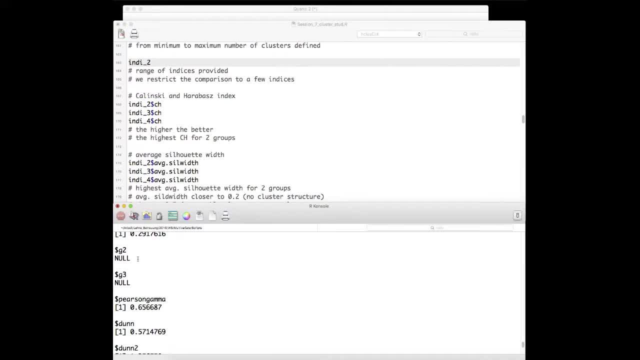 discussed before. If you set options to true, it would also calculate some different indices and so on. There are many different indices computed here. We restrict our focus on the Kalinske and Harabas index that we have discussed in lecture, so I don't go into details here. Just keep in mind that this 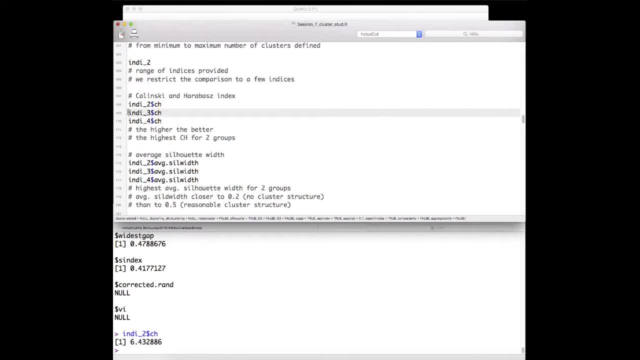 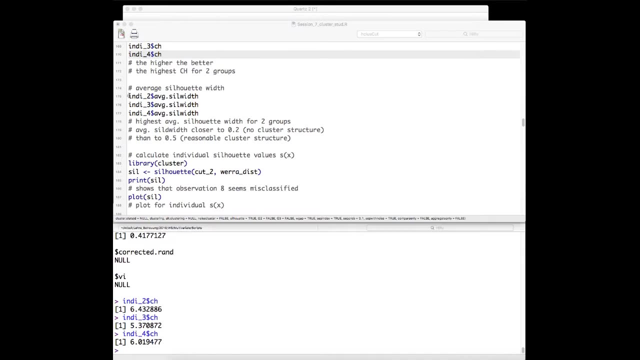 index is based on sum of squares, and the higher this index is the better. So here we see that we obtain the highest results for two groups. so we would evaluate. the two groups are the best solution for this data set. Now we calculate or we extract from the 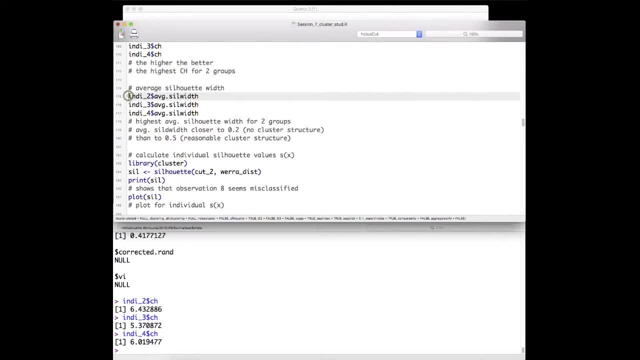 object: the average silhouette width. so remember in the lecture we also discussed that highest average silhouette width is the best, would be the maximum silhouette width indicates the best number of groups. the optimal number of groups. That would be again two groups here in this case. Also remember that 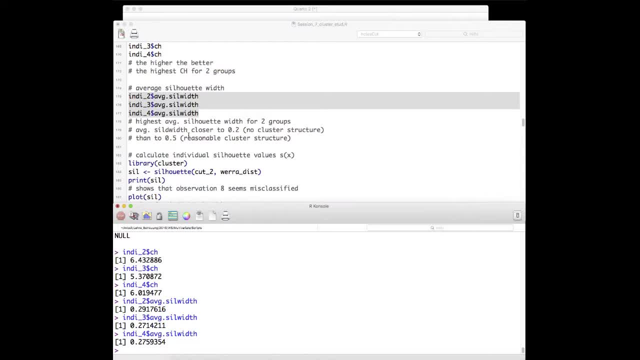 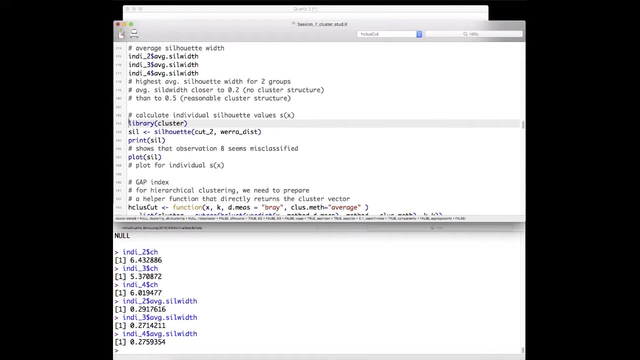 we had some kind of rule of thumb to evaluate the absolute values of the silhouette width, and it would be: for 0.2, you have no cluster structure, and 0.5 means you would have a reasonable cluster structure. You can also calculate the individual silhouette values and remember that this gives. 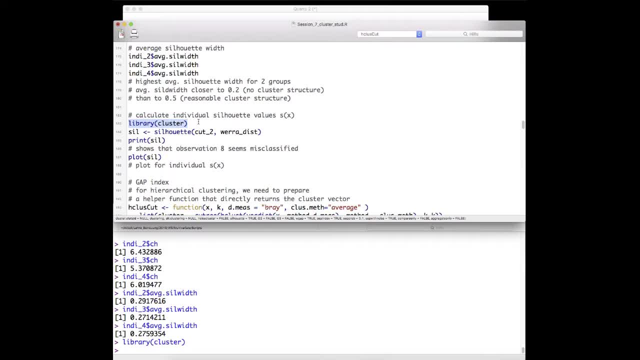 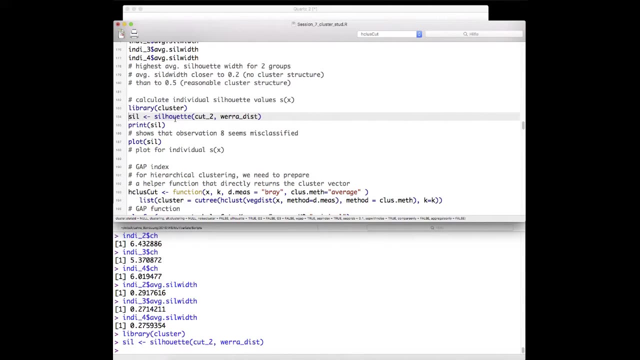 you the average distances within the cluster of an individual observation and to the nearest neighboring cluster, and negative values indicate that the observation might be at a better place in another cluster. The silhouette function you just provide, you just provide here the resulting clustering and the distance matrix. 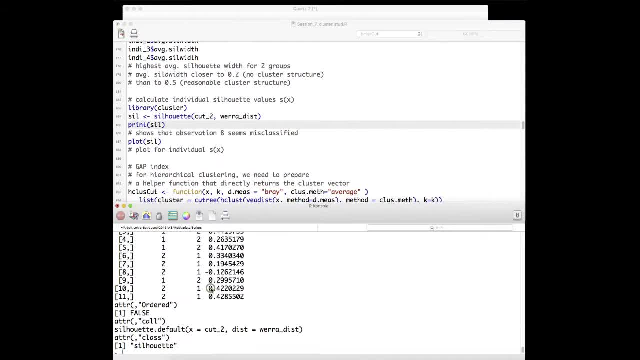 and then you obtain the results for each individual object and we see that actually one of the sides is supposed to be placed or, according to this index, has been placed in a cluster. so the silhouette width is minus 0.12. so observation eight might better be placed in another cluster. We can also plot the silhouette. 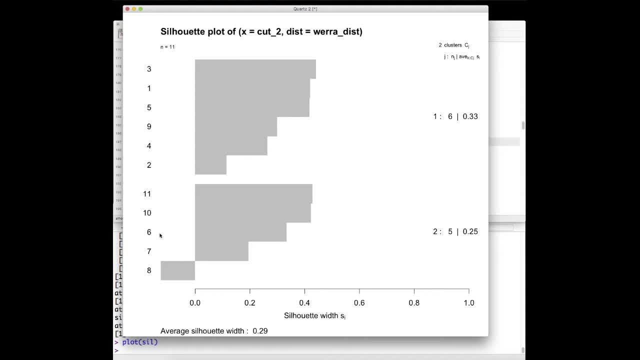 width. so it shows us the values and the values for each side here in a graphical display. This is cluster one, this is cluster two and these are the average silhouette width. So according to this plot we might better place this observation, the side eight- into cluster one. 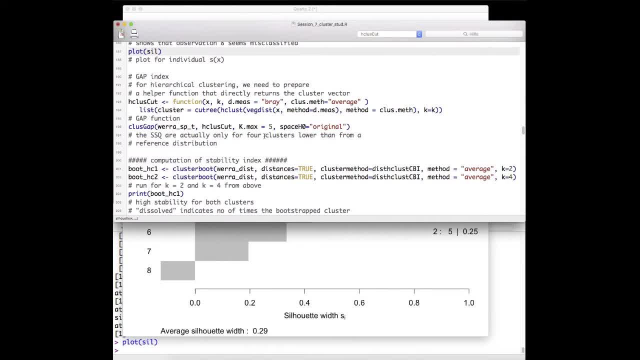 And finally, we calculate the gap index. Remember that this compares our data to a reference distribution or from the same data. Now, remember as so the gap, the cluster gap function is initially tailored for k-means clustering, but we can make it work which with hierarchical 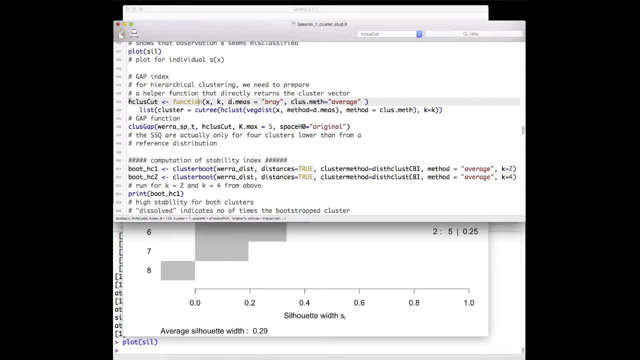 agglomerative clustering, but we need to define a function, before which then this is done here- h class cut function which in the end runs the hierarchical agglomerative clustering and directly cuts the cluster. the dendrogram, at a certain point to that will reside in the desired 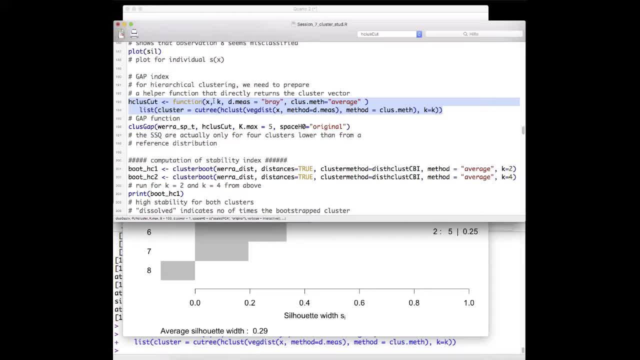 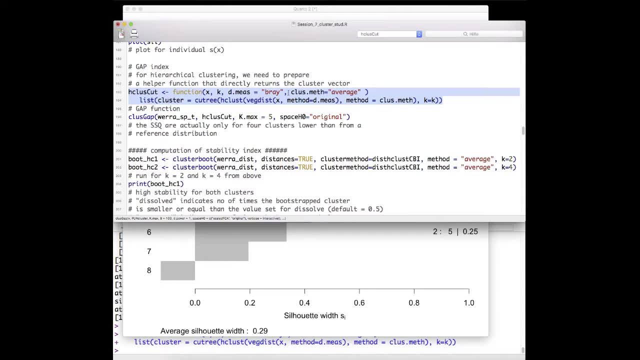 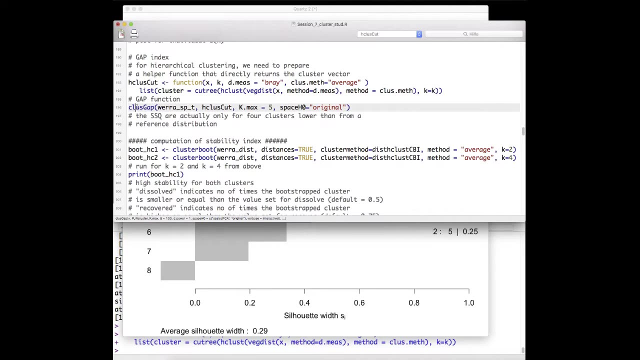 number of clusters. We don't need to explain that here in detail. have a look into the individual clusters. So let's look at the cluster gap function. We can see that the cluster gap function is actually a function that calculates the number of clusters that are nested here within looks a. 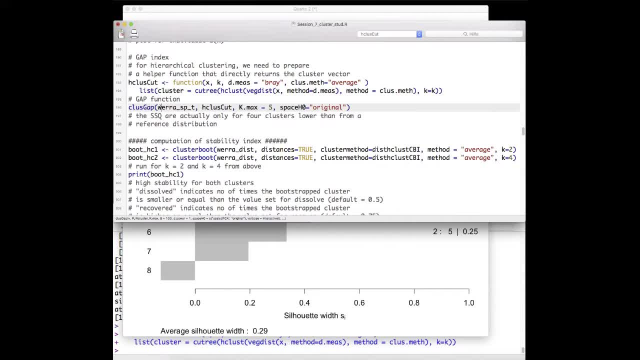 little bit complicated. That's just a helper function so that we are able to calculate the gap for hierarchical, agglomerative clustering. Now let's look here: The cluster gap function: you provide the data, you provide the function that calculates the cluster, the clustering. then you provide the. 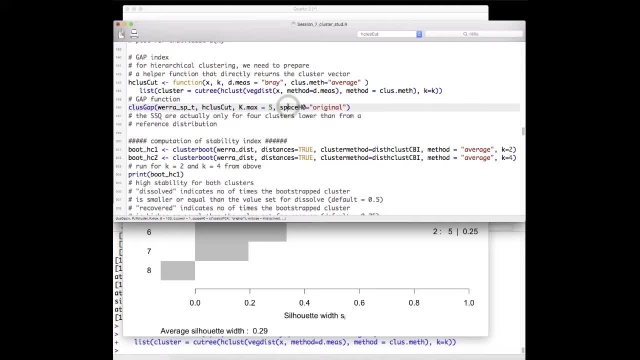 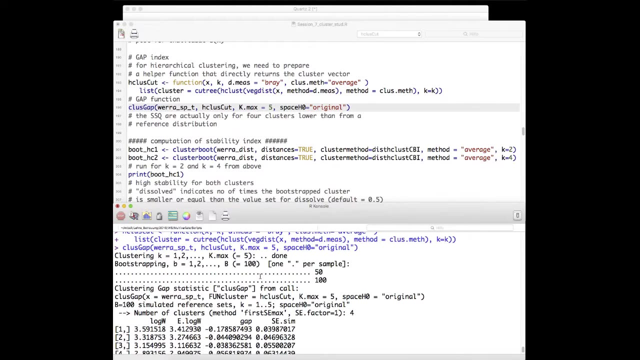 number of clusters that are nested here, and you provide the number of clusters that are nested here. So the cluster gap function is a function that calculates the number of clusters that are nested here. You also provide the space from which the data is taken for the reference. 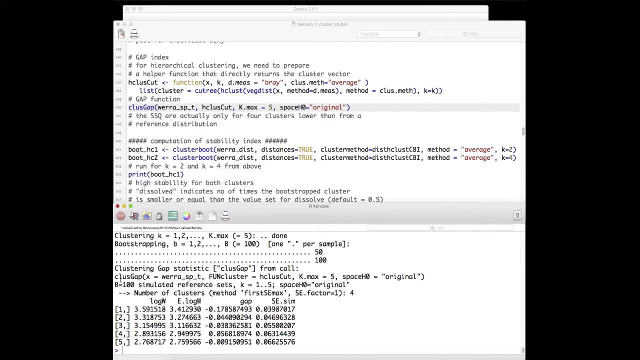 distribution. so we take here the original space for the null hypothesis. What do we obtain? We see that there's bootstraping done on the original data for five data sets and we obtain then we have: we see here that it also gets the number of clusters that we need. 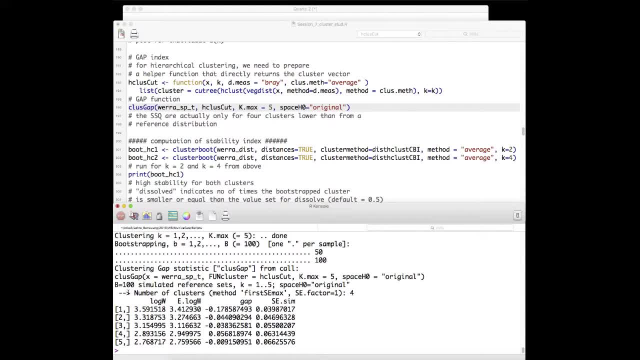 gives us this judgment on whether we- which would be the number of clusters that results in the largest gap, and that's actually done here- based on the first sum or difference in the standard error that yields the maximum difference. so it's not the absolute maximum, but it's the opposite: it's the difference. 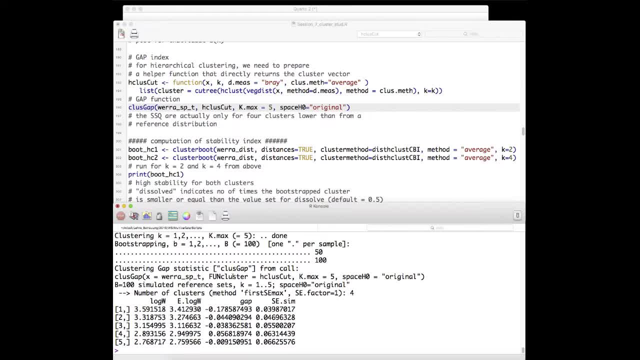 between the reference and our data, and that falls within one standard error. so we can also modify this standard error. you could choose also just using the maximum gap value. if we look at the gap values, we see here that indeed the gap value is lowest for for as high as for cluster four. in fact, in all other cases our clustering 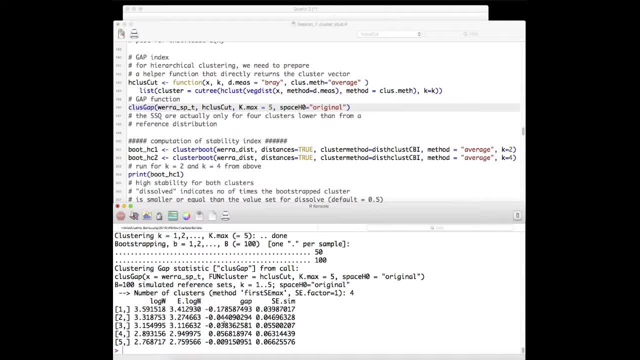 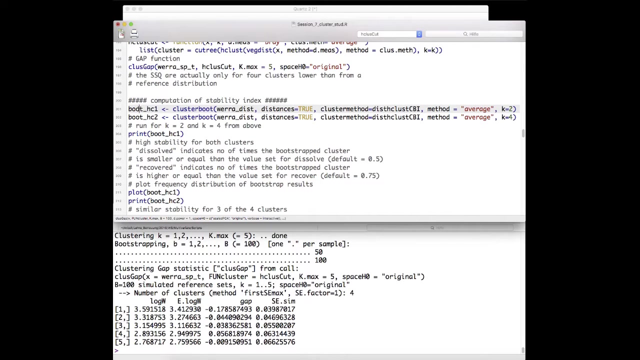 result is worse than that from a randomly drawn reference distribution. so you could evaluate that the clustering is not particularly good for this specific data set. so so we decide we should decide here on four crews. based on this we can also calculate the stability that's done with the cluster boot. 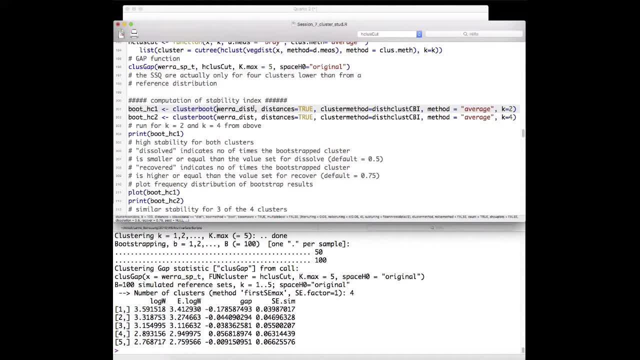 function- cluster boot function- takes again as input here, if you have the distances calculated already, you provide the distance matrix. you set distances to true. you have different clustering methods that are used for which you evaluate the stability. have a look into the help for the function. you see that it it's very versatile. it allows you to define many. 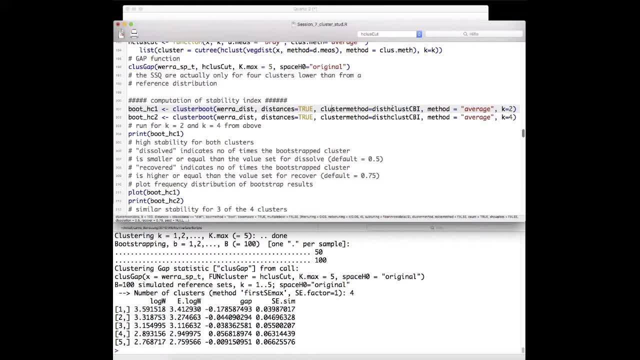 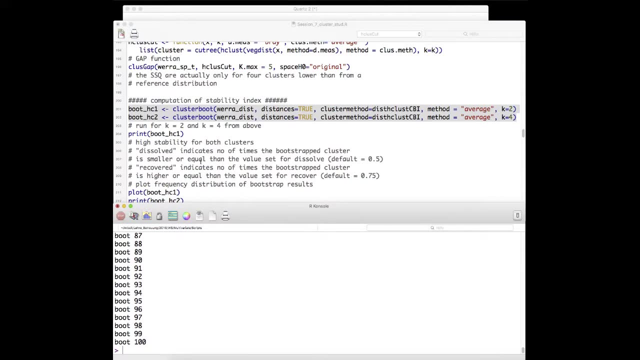 different methods. from K means two different hierarchical and collomerate of clustering methods and here the clustering method, the average linkage clustering, and we calculate the stability for two and four groups. so it takes bootstrap samples and we print the results. we see that here we have a 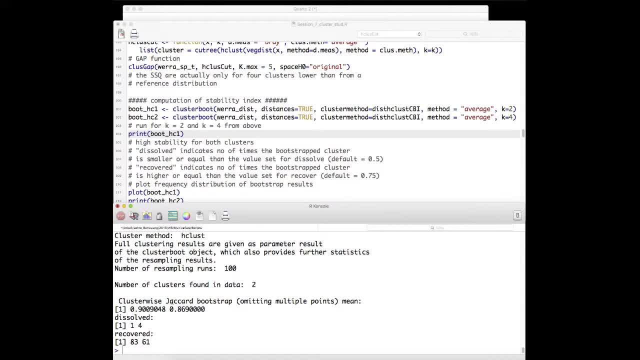 here the clusterwise jacquard bootstrap results in the mean jacquard index. so it always compares the bootstrapped, the bootstrapped data to the original data in a pairwise manner and calculates the jacquard index. so how much we have? how good is the match between the different data sets? 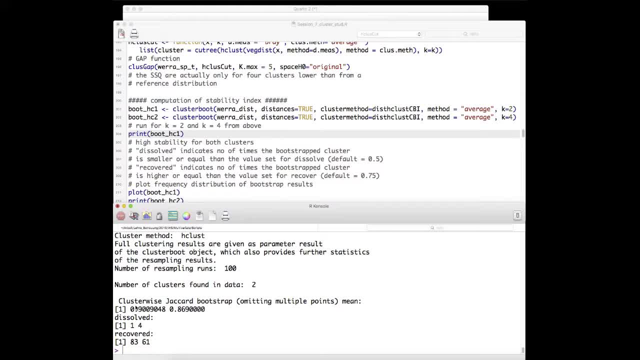 we see that the average match in terms of the jacquard index is very high. we have a mean of 0.9 and 0.87. dissolve means how many times our our jacquard index, for pairwise means, fell below 0.5 and how often it was. recovered means how often was above 0.75. so you can set these. 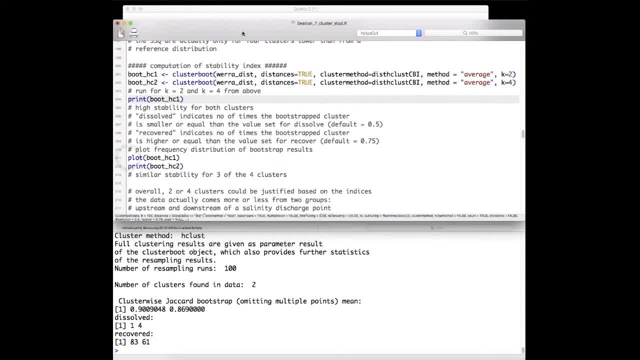 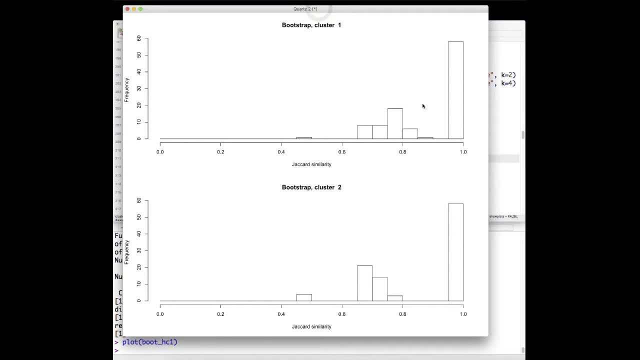 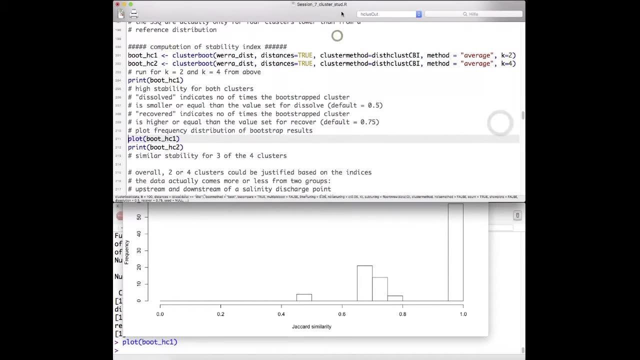 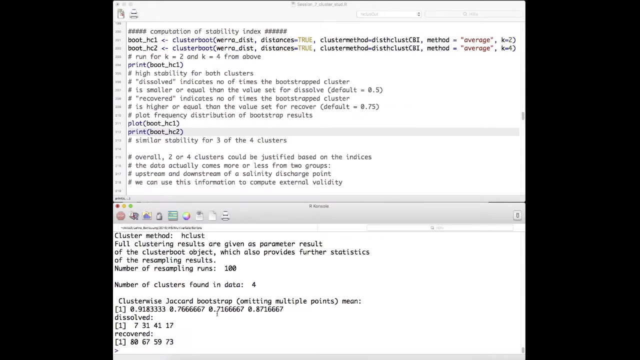 thresholds according to your objectives as well, so we can plot the results, the distribution of the pairwise jacquard similarity for the different bootstrap samples and, yeah, have a look. if you look at the stability for four clusters, we see that most of the stability values, the mean jacquard values, are below the values for. 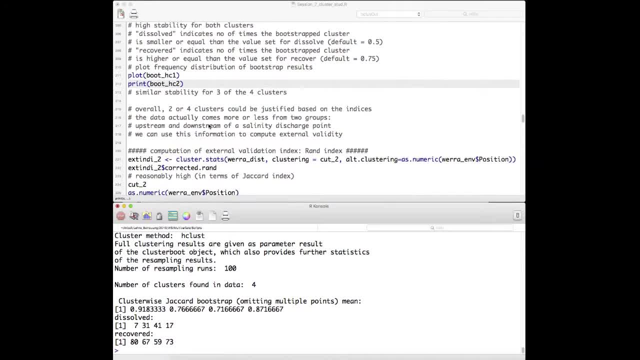 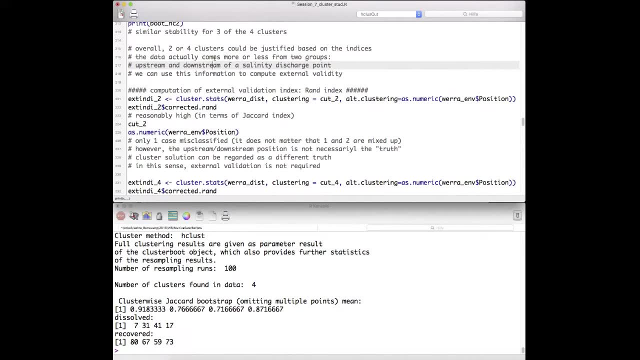 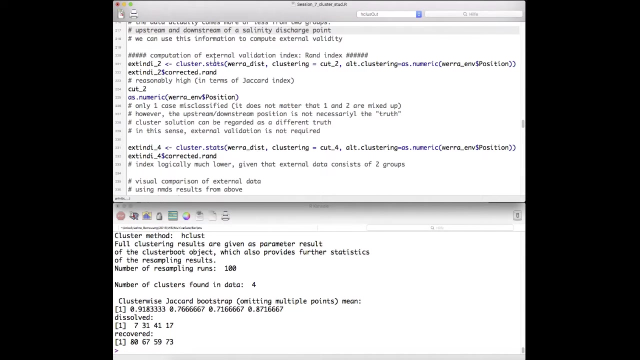 for two groups. so two groups seem more stable than the solution with four groups. overall, you see that, depending on the index and on your aim, two or four groups could be justified. based on these indices, we finally calculate an external validation index, that's the rand index here. so the rand index is uh calculated by the number of data sets. you'll see. 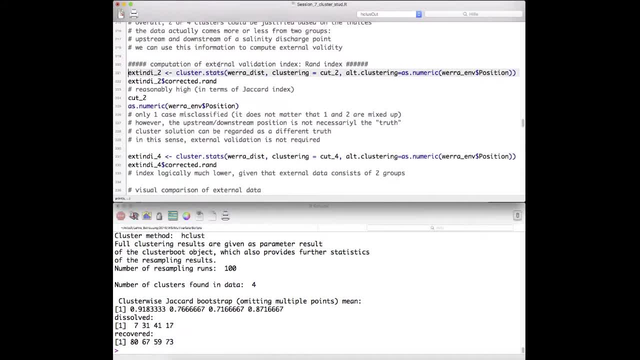 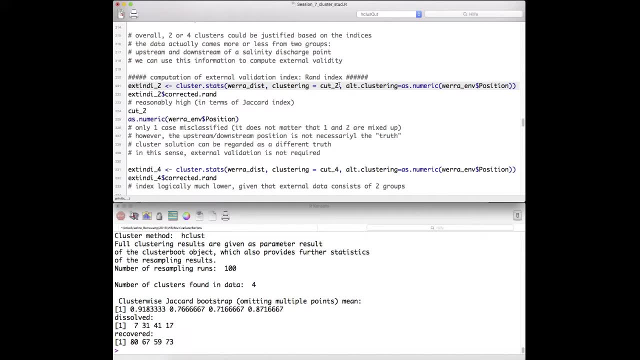 it also with the cluster stats function and the cluster stats function. we have used already the changes here that beside the clustering provides our initial clustering. we provide as alt dot clustering a numeric vector of the grouping structure that is used for external validation. so that is used as. 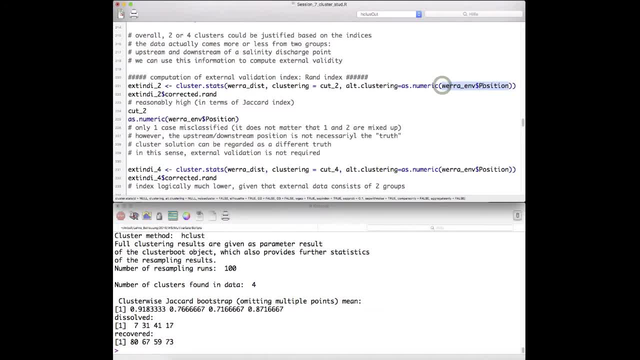 so-called ground truth. remember, if we look into this, this is a, this is a factor with downstream and upstream, and we need numeric vectors, or by using the function as numeric on this, we have the result that we have twos and ones as integers in this vector, so we can calculate. 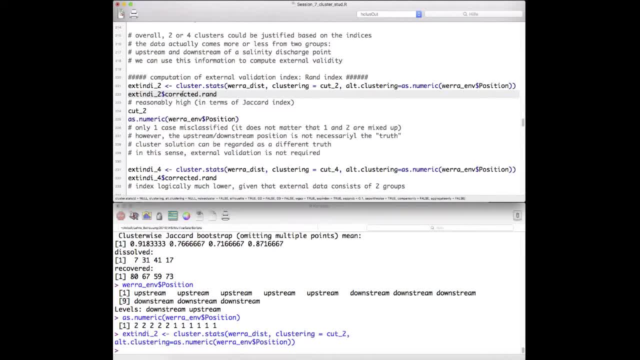 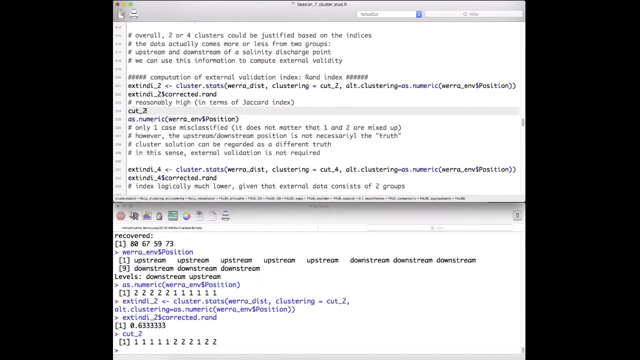 the cluster stats again, so we would obtain all internal cluster indices as well. and then we extract the rand index and we see it's point six, three. so that's reasonably high. keep in mind that it's also similar to the jacquard index, that has been to the similar matching coefficient as well. have a look into the. 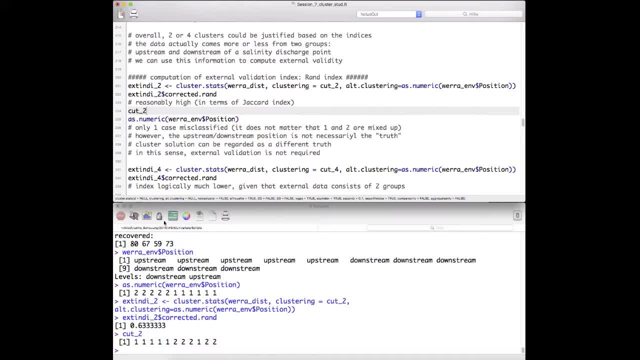 have a look into the lecture how this is calculated. note actually that if we would look into the data you would see that we all only have one of the objects misclassified. so you see here that misclassification of just one of the points results in reduction, quite some reduction, in the adjusted rand index. you will later on see. 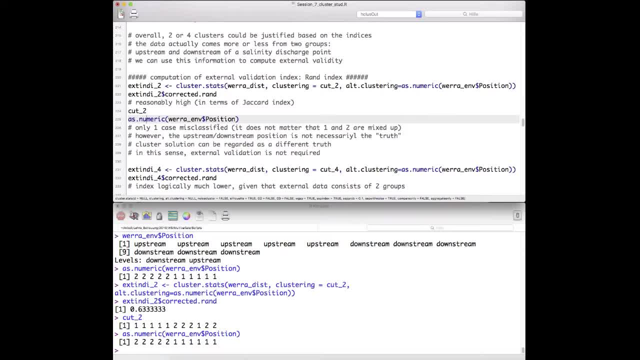 that for a data set with much larger sample size, that this reduction is much smaller and we can compute this rand index as well for four groups and we see that's actually much lower. that's not surprisingly, because we have external data with two groups. now if we have found four groups, then it is obviously 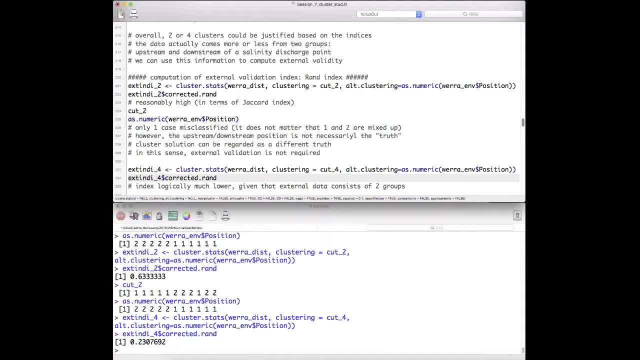 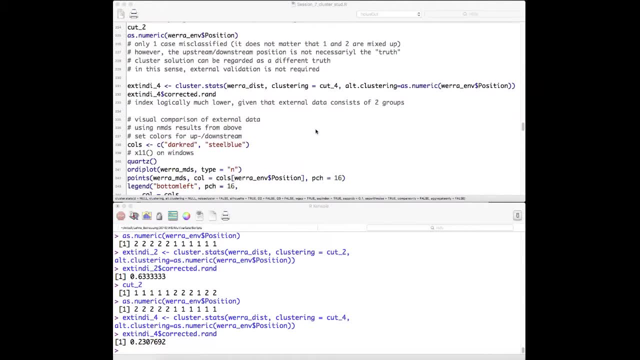 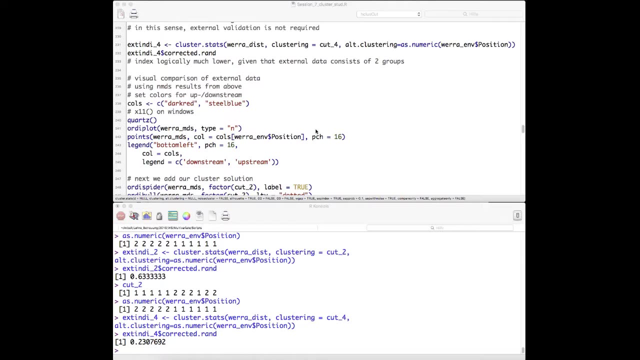 worse fit. now, a different way of comparison with external data is to just visualize this and, as you remember, we just used NMDS for visualization and that's what we will do as well. we select colors here for the external data, so dark, red and still blue are assigned. we will later assigned to the upstream and downstream. 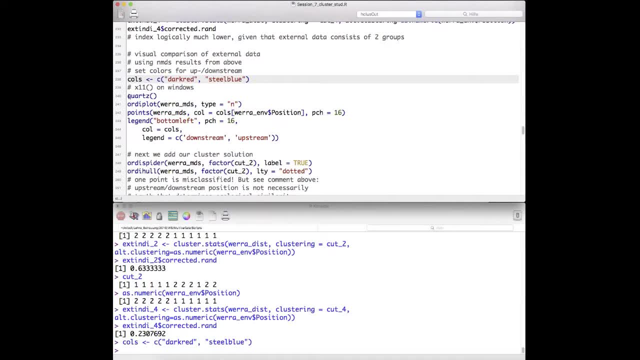 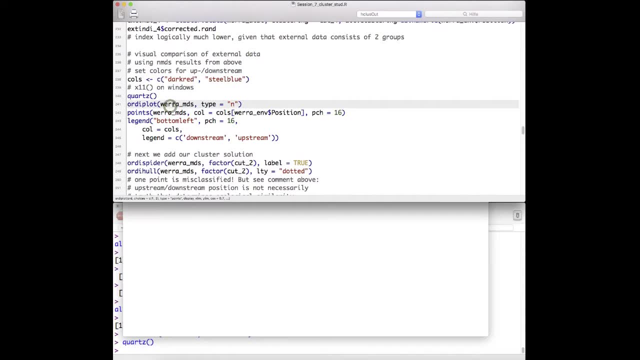 position and then we open a new graphics window- that's x11 on windows, and we plot again. that's the same. it's more or less the same code as above. the only difference is that we have the color command here and the colors are given by the vera position vector. so 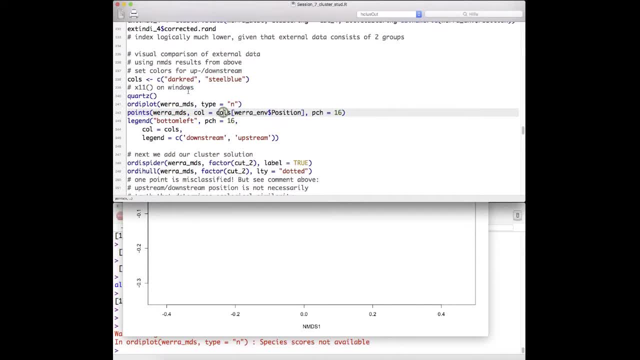 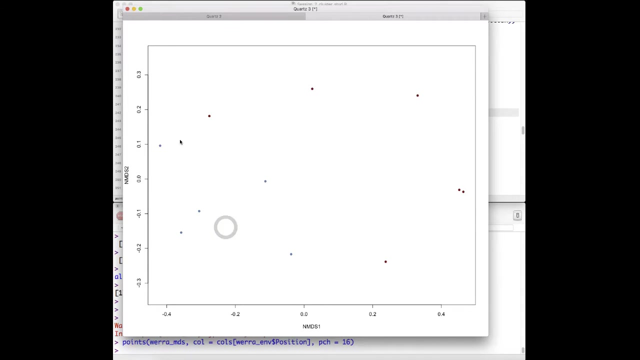 remember that's a factor. so we say that the positions of this color vector are selected based on the factor that is provided in the vera position vector. so how does it look? how does this look like when we plot this? we now see we have blue dots and 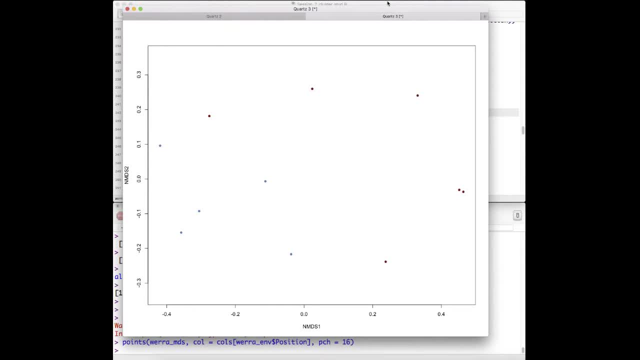 red dots. the blue dots are related to the upstream sides and the blue dots are adjacent andEuropean assets down in blue, which is the respective position. and blue dots are related to the upstream sides and mourning tissơi dot Dual Ansch drove on them also, Gym那. 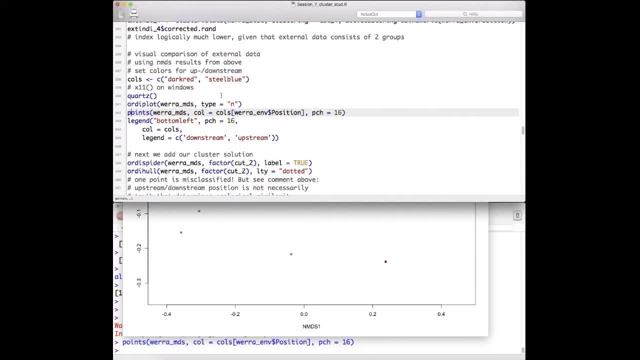 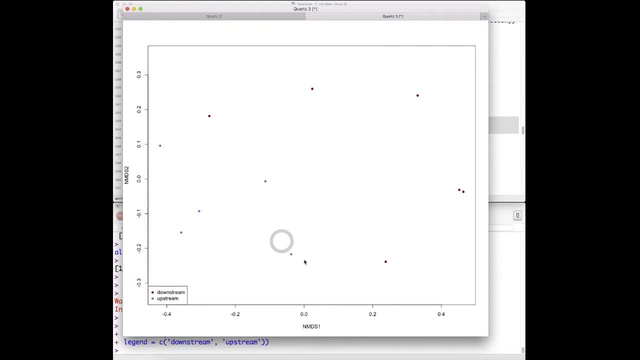 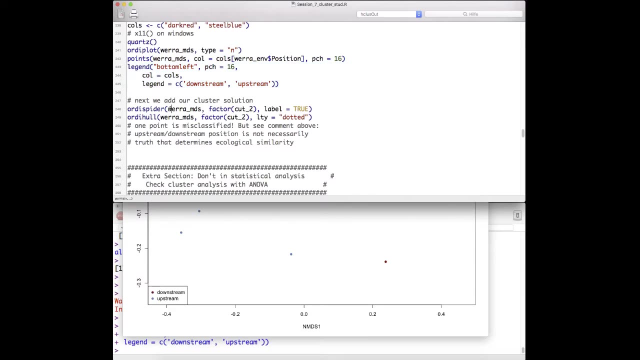 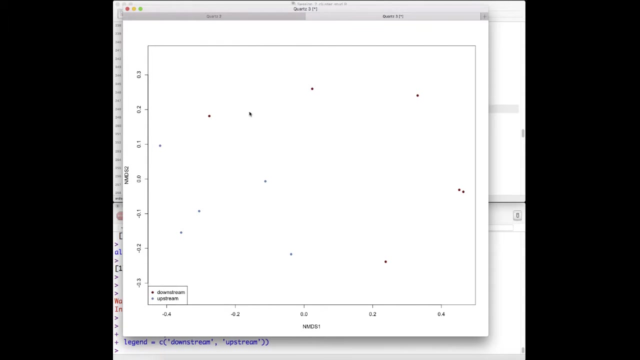 are related to the downstream sides and the others to the red, to the upstream sides, or maybe conversely, red is downstream, blue is upstream sides. now we add our, so this is the external data. so this shows you to which position along the river gradient the sample belongs to: the clustering. now, this is the original data as well: the clustering. 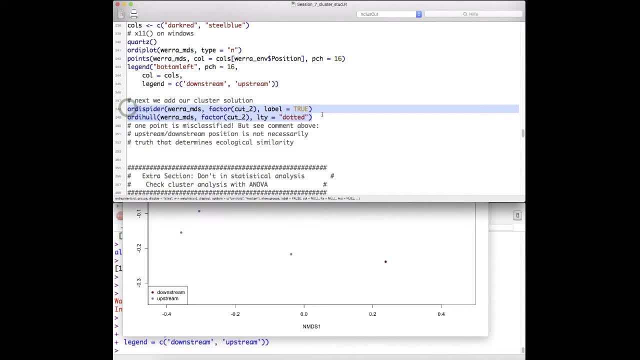 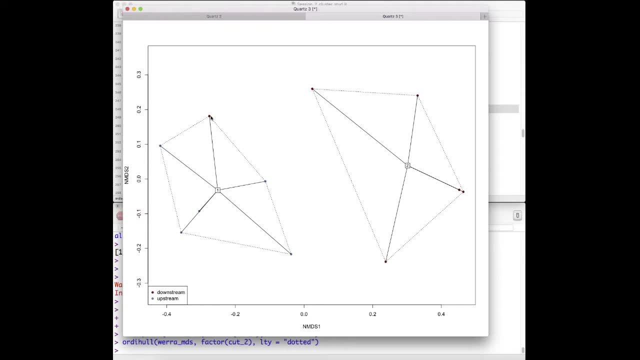 now assigned these different points to clusters and we plot the hull and the spider as above and you can see here visually that this red point here is certainly misclassified and that's the point that we have already misclassified according to the external data. so we might. 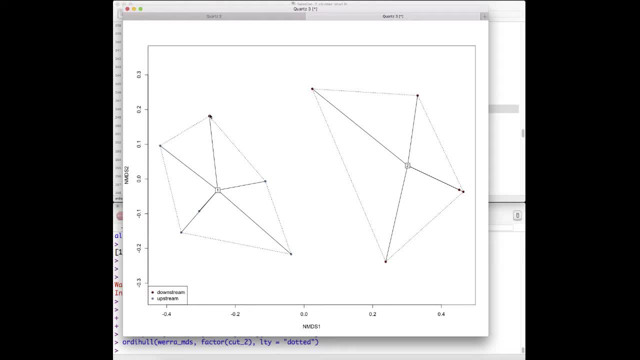 evaluate that this, that this uh point should belong to the second cluster based on the external data. they turn into the external data. that's a downstream side, but it's characterized at upstream, so this also teaches us somehow that we can't 100 rely on the external data, because the 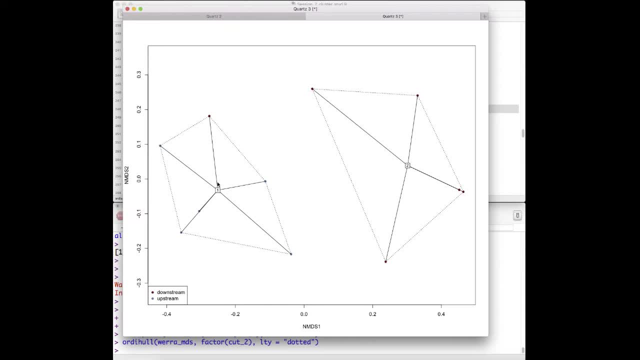 so-called trown truth is the ground truth with respect to the geographic position here. but is it necessarily the ground regarding the ecological groups that we find in the rivers? apparently not, obviously not. so we have certainly the putting or or assigning this observation, this species composition to group, to the group, to the first group here makes more sense and the ecological 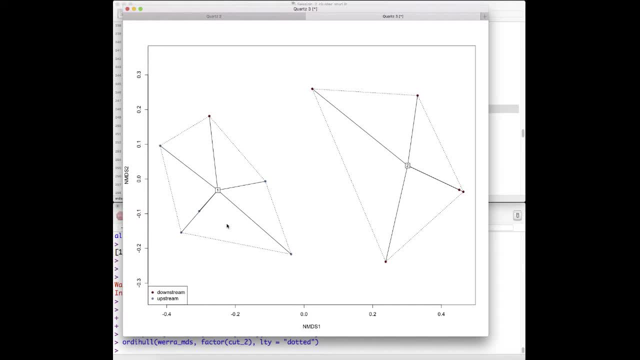 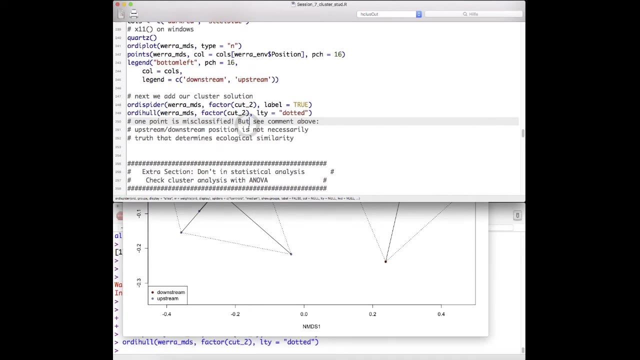 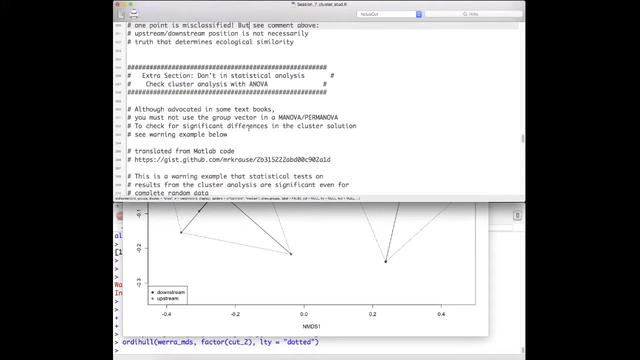 interpretation or explanation maybe straightforward. we, it's most likely the case that in this, although it's a downstream position, in this position, the effect of the discharge has not hit yet. so here you have a, an extra session that shows you one issue. it's- and this is in some 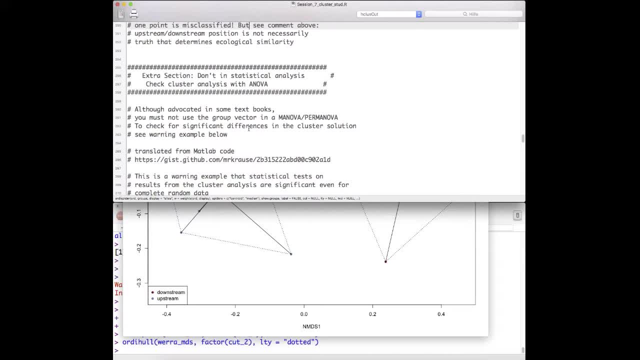 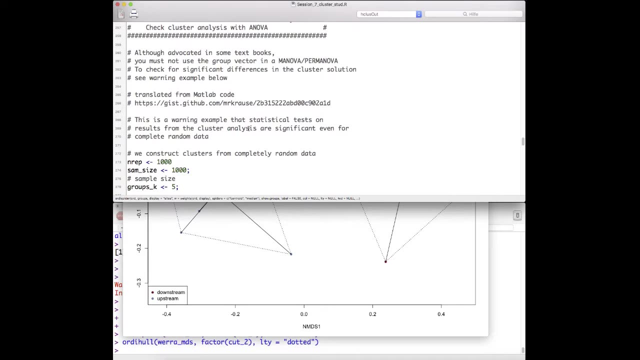 textbooks you read that you can do a cluster analysis and later on check. you can do a cluster analysis and later on check results via anova, and this should not be done and this warning example shows you that just using random data, putting this into a cluster algorithm, you will find some grouping structure that is 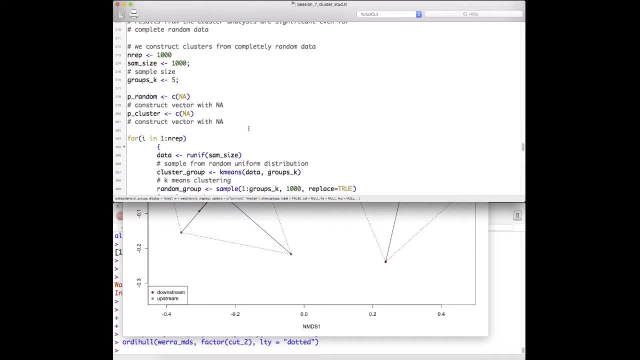 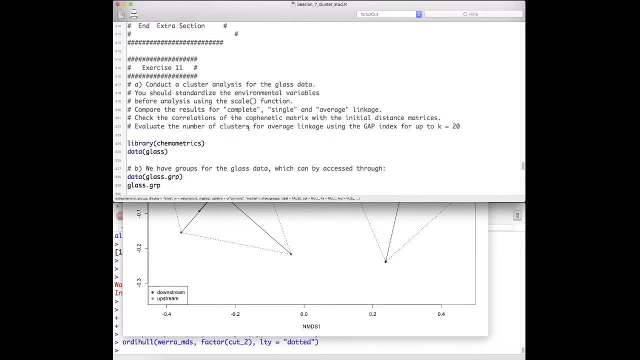 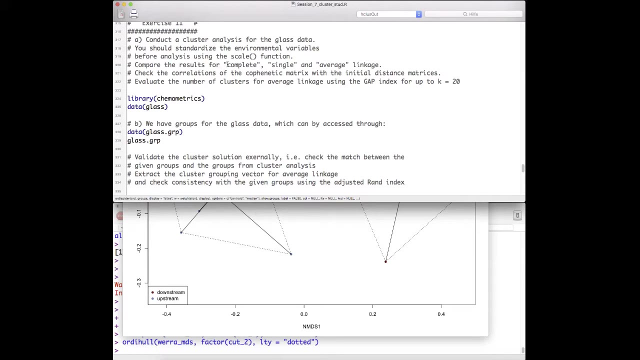 statistically significant. although that makes no sense, i'm not executing that. that's rather an extra session for those that are interested. so have a look, okay, if you're interested in that. and then you have the exercise here where you should compute, we should. you should run for a. 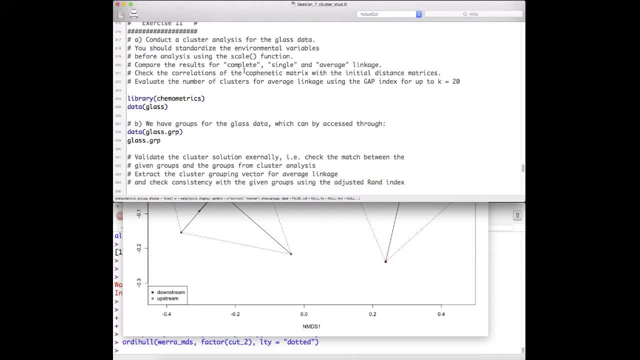 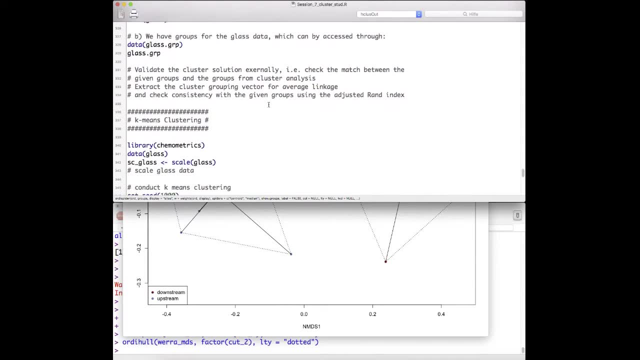 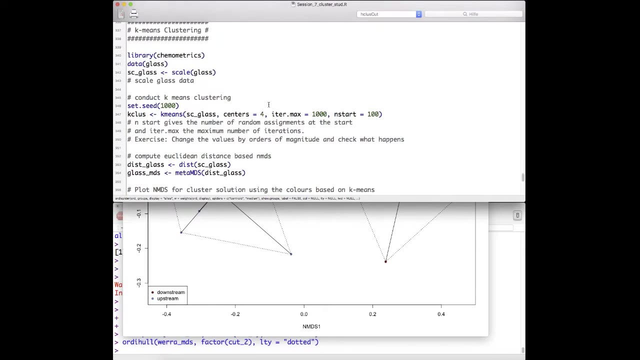 new data set, the complete single and average linkage, hierarchical clustering analyzes and a couple of other things that are described here in the text. so have a look. you will find the solution to this answer to this exercises as well, provided on the website in a few you weeks. 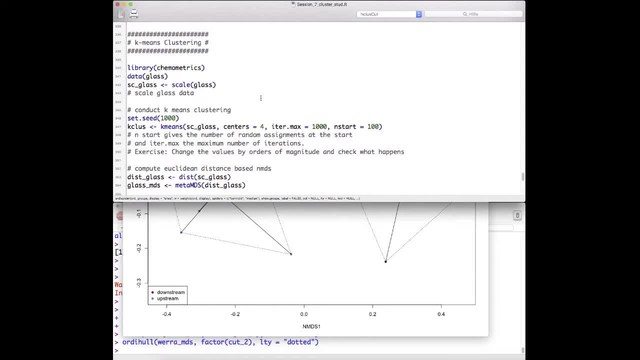 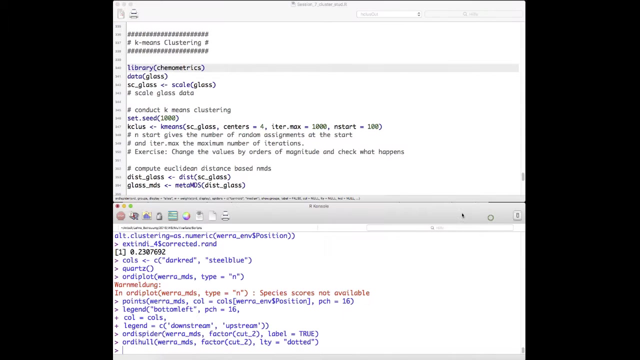 now. we have discussed extensively the hierarchical acclomerative clustering we have to. we know that in the lecture there's also non-hierarchical clustering and k-means is one of the widespread clustering techniques in use for non-hierarchical clustering and we illustrate here how you can use k-means for clustering. remember that for k-means 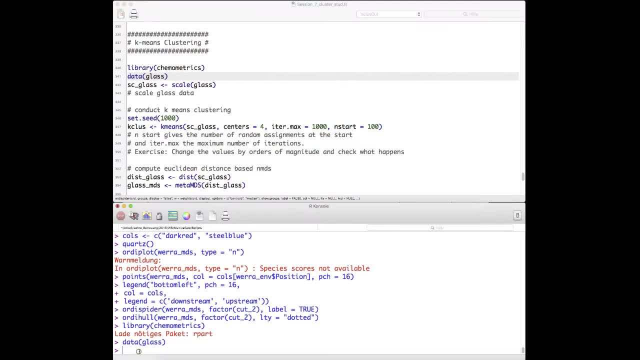 as well. you can use k-means for clustering and you can use k-means for clustering. for clustering as well, we don't know what is the, what is the number of groups, and we need to provide the crew number of groups before, so that's something that we didn't need to do for the hierarchical. 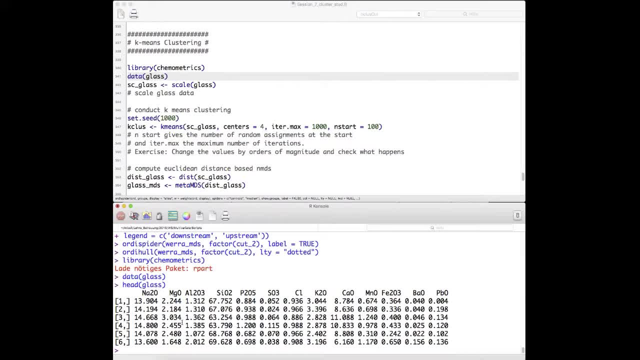 acclomerative clustering. looking at the data set that we load here- the class data- you see that we have here. this is actually the cloud that the data set are class vessels that have been found in different places and we have to provide the crew number of groups before, so that's something that we 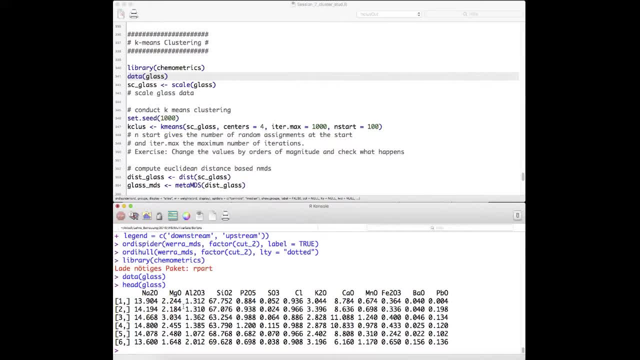 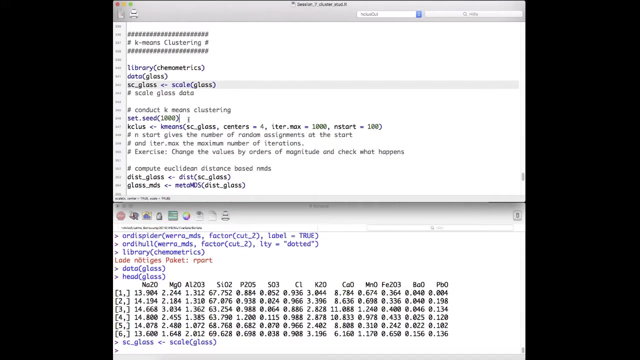 different locations and there have been the the iron contents. different different minerals have been measured in these classes. so we scale the data before. we can already see that, for example, silicon dioxide has much higher values concentrations than so3 or chloride. so we scale the data to have the same mean and variance and for the k-means the function is just. 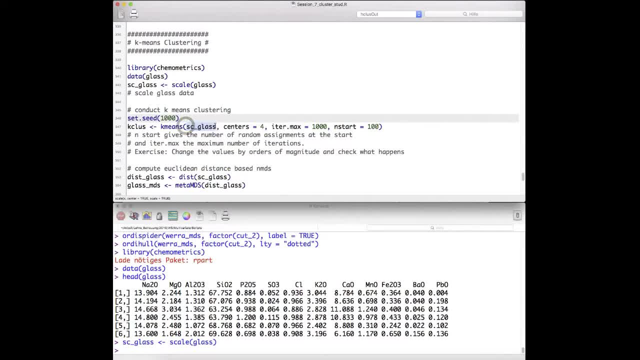 called k-means. you provide the, the data. so here the scaled class data set. you tell the function how many groups you want to build. so that's the k that's provided as centers here, and then you have the number of stars. so remember that we have the number of stars and we have the number of stars. 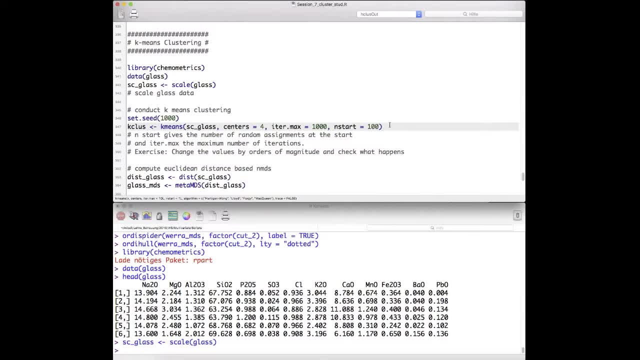 here that the material humble there. if I do go from this willounding cost you the number of stars to this is equal to that himself. you get different values, energies, anything fundamental behavior for this cell isger and function along here. so let's take that function here. that's already. 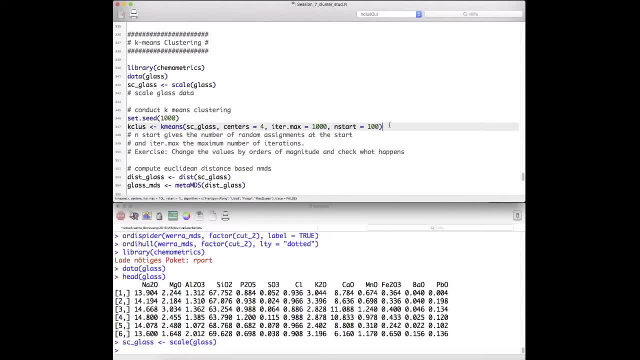 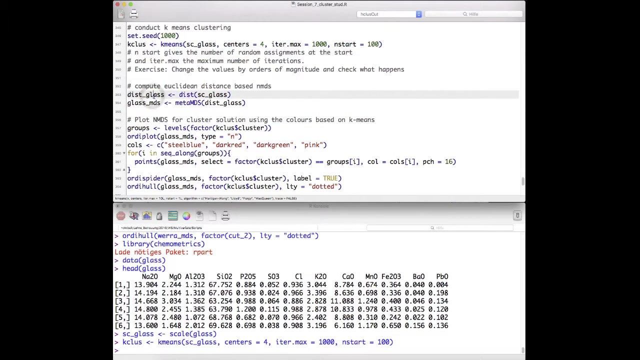 executed. so that's the. so in this example. here the the aggregate mass of egg %, and that's much higher here. so here it's much higher. but we wouldn't otherwise get such a big of points and that's why we do several starts. So we run this function and we 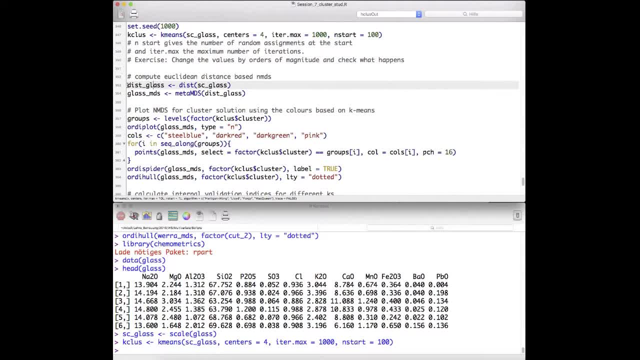 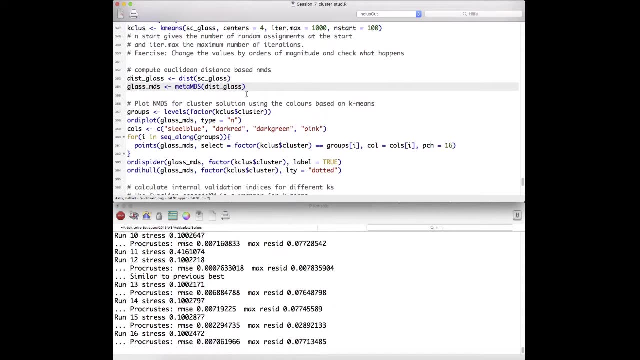 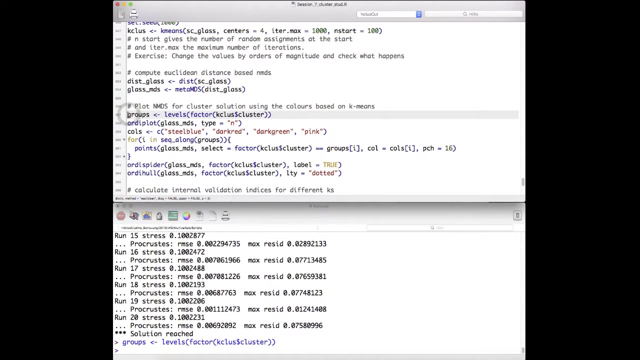 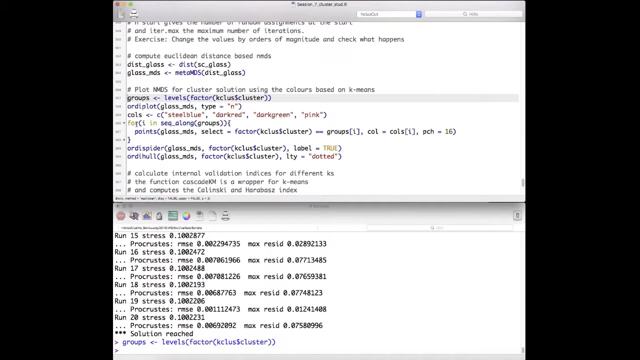 display this function later on. This has been done before. so we calculate the Euclidean distance, we calculate the NMDS and we display the result. So that's something we would call external validation. We display the result against the NMDS here, So we choose different colors. So again, we first use ordiplot without. then we 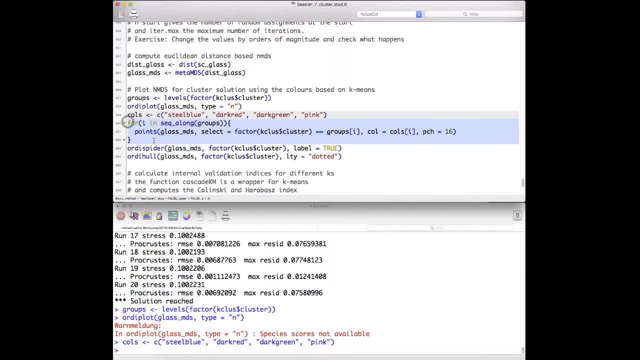 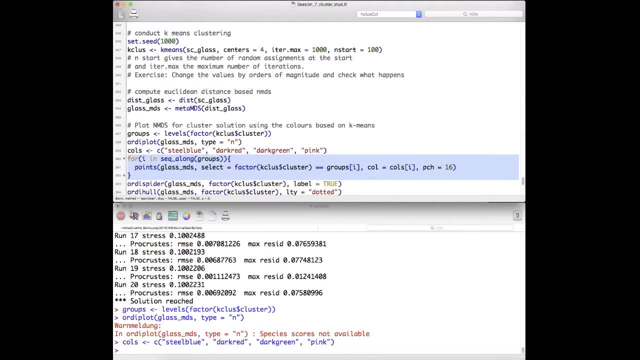 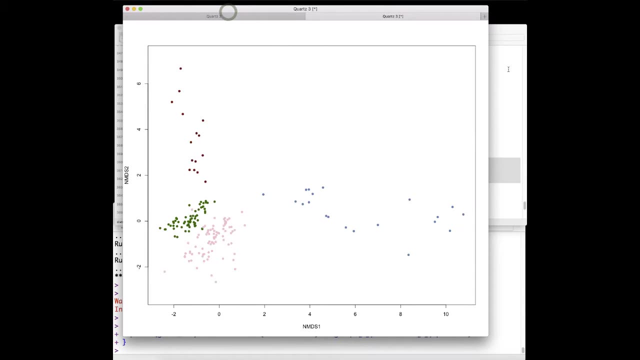 select some colors that we want to plot and we choose the color that we want to plot. So we choose the color that we want to plot and we plot here then the points of the of the different clusters. So remember, we have created four clusters. here Again, this looks like that, this one, Interestingly. 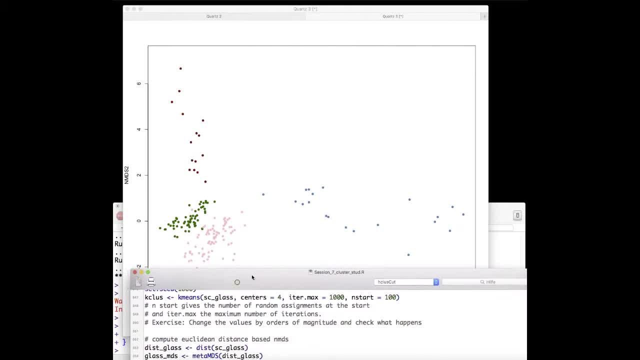 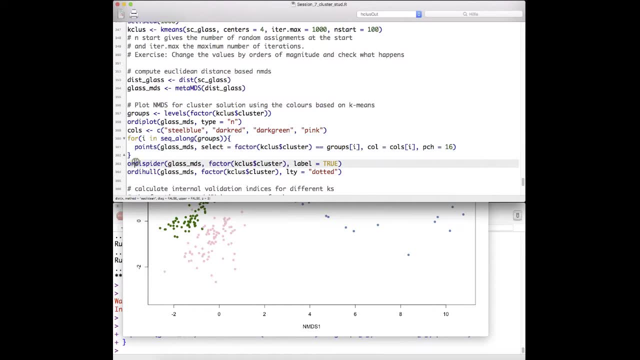 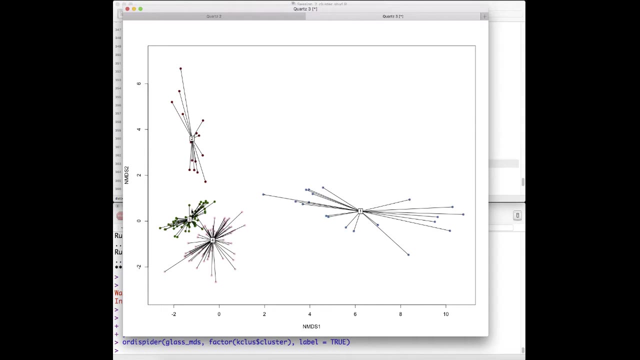 this point looks clearly ill assigned. It seems to be an error here. You could theoretically, after you extracted the partitioning, you could theoretically see which point that is and assign this point to cluster three, for example. Apart from that, the clusters look reasonably separated, Although we could argue that three and four 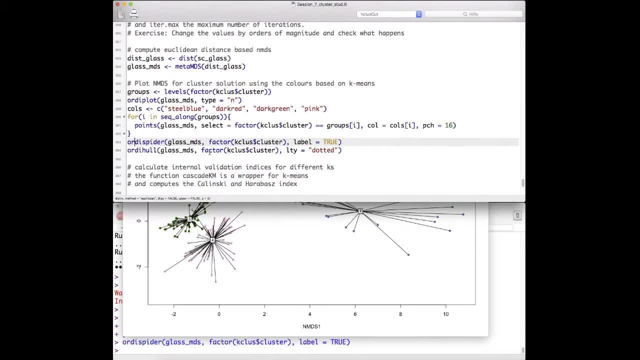 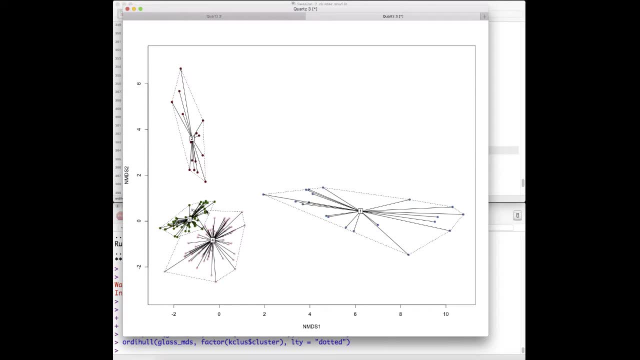 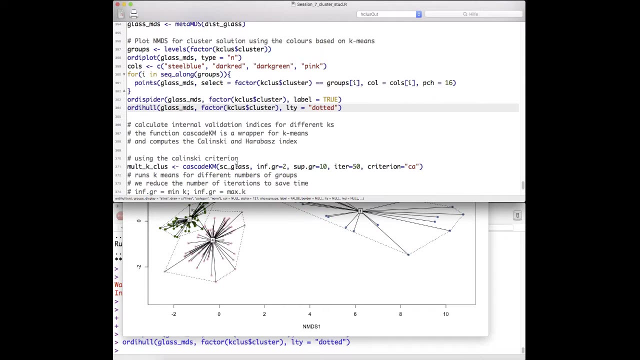 could be merged into one cluster. So running again with three clusters may. So you see, here they are actually overlapping. because of this point The hull is overlapping. We can now calculate internal validation indices. We've done this above, So you have to adjust some of the 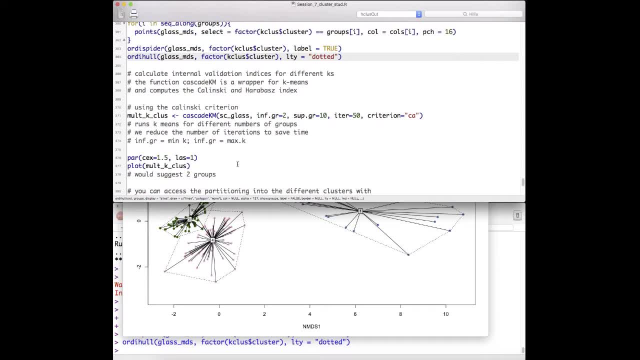 functions that we used above for the calculation of internal indices, depending on which function it is, and provide the function, the information that we use here k-means and not a clustering. One function that has been created specifically for the clustering of different groups is the cascade KM, and cascade KM allows for the 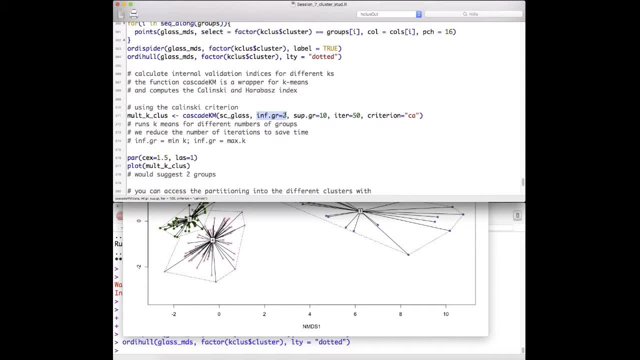 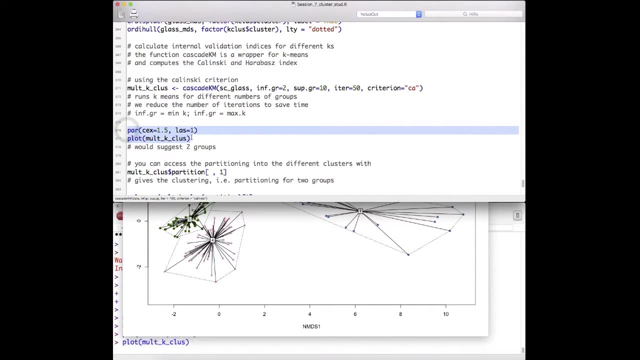 given data set to calculate the Kalinske criterion. You could also select another criterion, but the Kalinske criterion for two up to ten groups. So we do this and then we can actually plot this And what you see here on the left side. 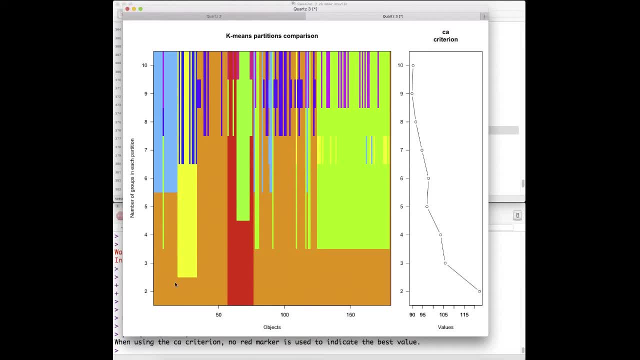 is, it's the objects where the objects, and you see here the, not the groups, the groups. in each partition you see here the number of colors tells you how many groups are assigned to which group an object is assigned. So you have here object one, for example, belongs to 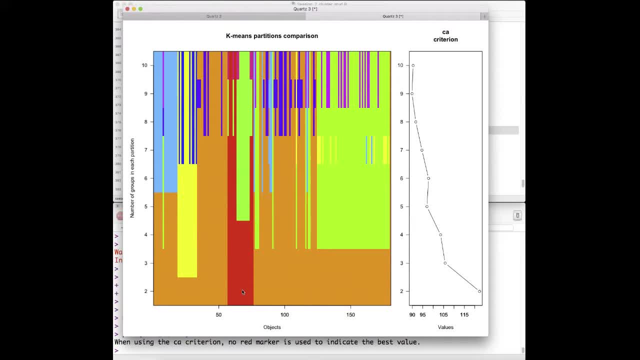 group one. we have just two groups in the beginning, group one and group two. then three groups are built and you can see which of the objects are belonging to the individual groups. So you go from bottom to top And you can read like a barcode almost. You can read here for one line Always you choose six or seven or eight, So it's obviously discrete assignments. So you can read to which object, to which cluster one object would belong to and how many clusters you would have, or the data is distributed. 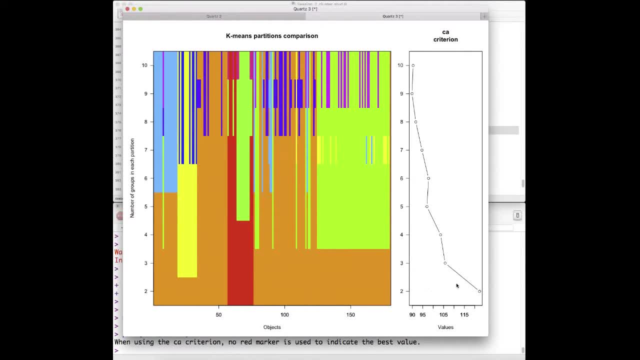 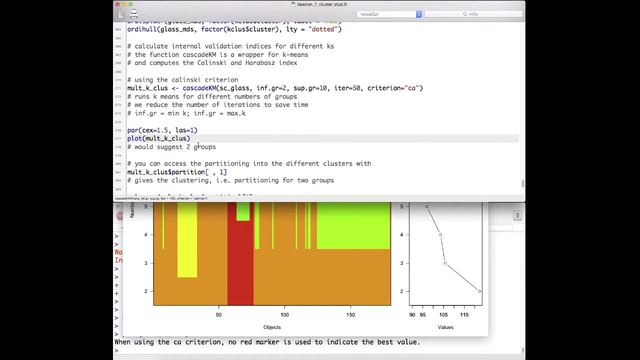 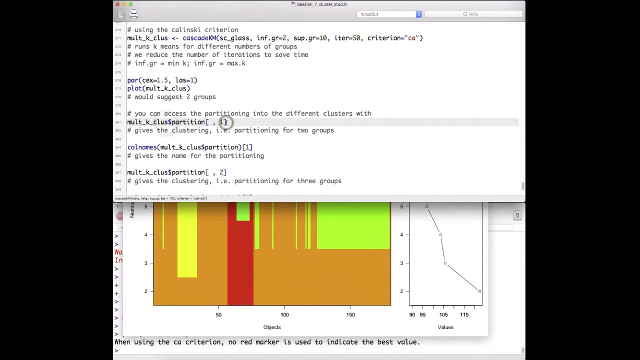 Here you see the number of clusters against the Kalinske criterion And you see the values for this criterion and that's highest for two groups. So it would suggest that we have two groups. here You can extract the partitioning into the different clusters, So the vector that assigns objects to a cluster with wire. 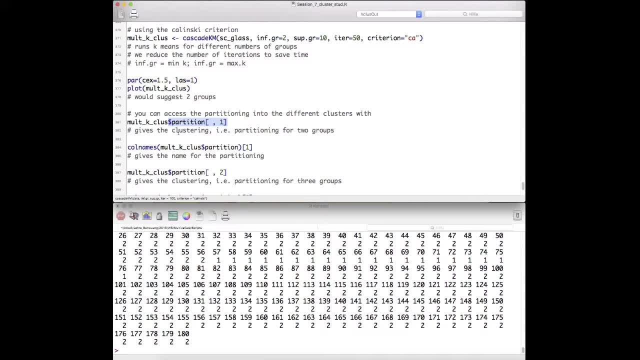 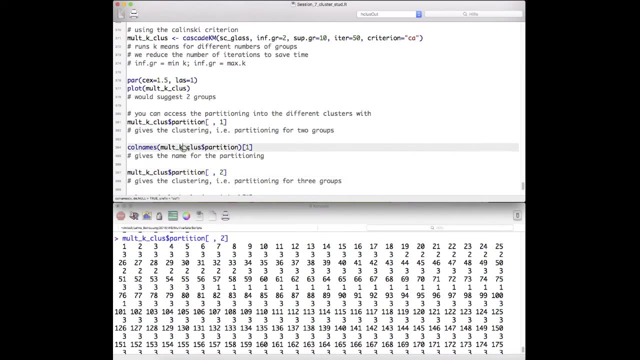 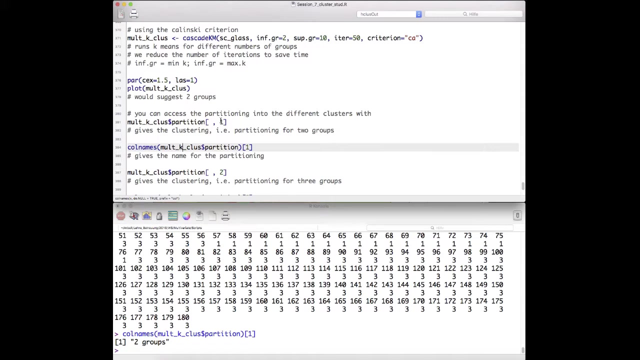 The partition slot. So partition one is the partition for two clusters. If you would use this function, you had the partitioning for three clusters And the call names. that would give you the confirmation that if you select the first column here or the first element of the vector of partition, 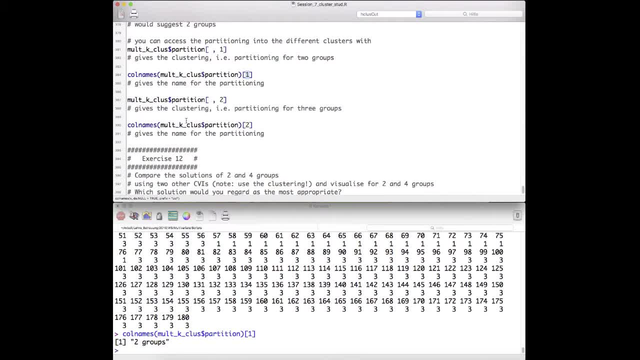 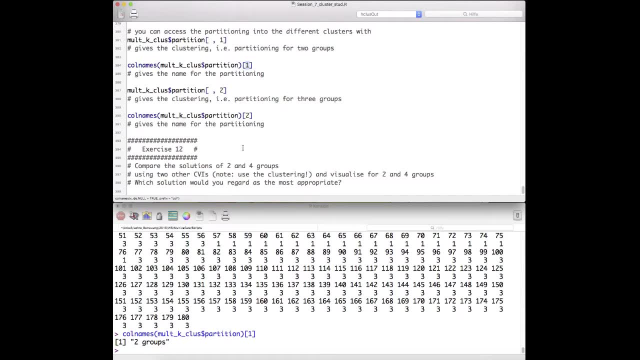 The first name would be two groups. So, based on this, we expect you to compare the solutions of two and four groups with two other CVIs that you can choose. Use the clustering. Use the clustering, So the partitioning, as input for these CVIs and visualize for two and four groups. 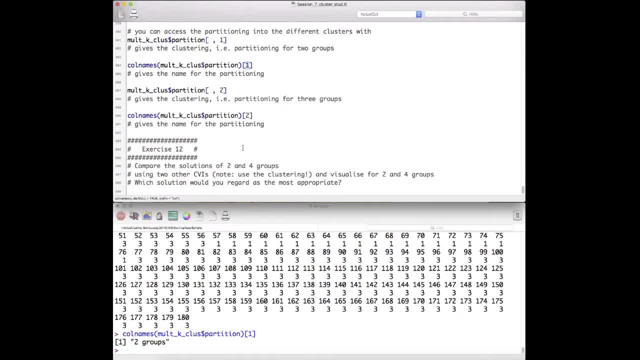 The clustering. Which solution would you use such a regard as the most appropriate? So that's it. I hope you learned something from this video and that is useful for your further work.